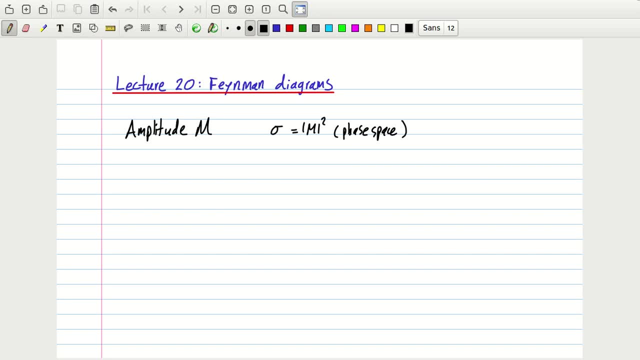 So these are the relativistic factors that guarantee energy and momentum conservation, but we still need to know what is our theory Like. how do different theories differ from each other, for instance? And all that is going to be in the amplitude part. So when we talk about amplitude- and actually I should use the word scattering amplitudes more specifically- I mean the quantum mechanical amplitude. 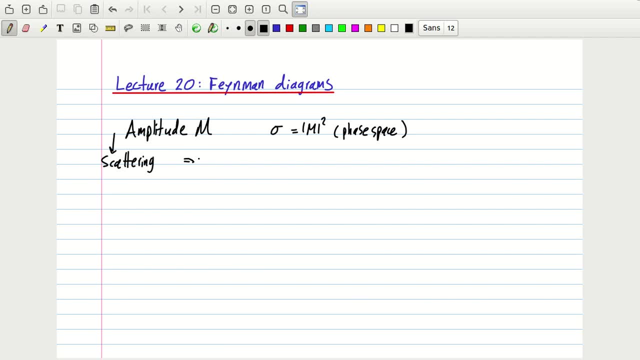 So it is a kind of transition amplitude in quantum mechanics. As you know, in quantum mechanics, for instance, you might remember that if you want to have an initial state, you might want to have an initial state. you might want to have an initial state. 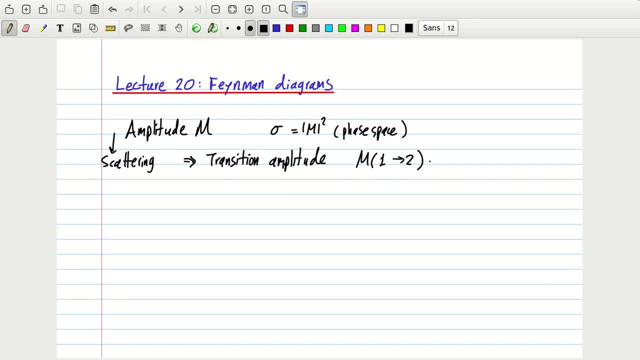 you might want to have an initial state and you go to a final state. Well, what happens is that you start from the initial state in quantum mechanics and then what you need to do is act with the Hamiltonian. So the Hamiltonian is what implements time evolution- right? 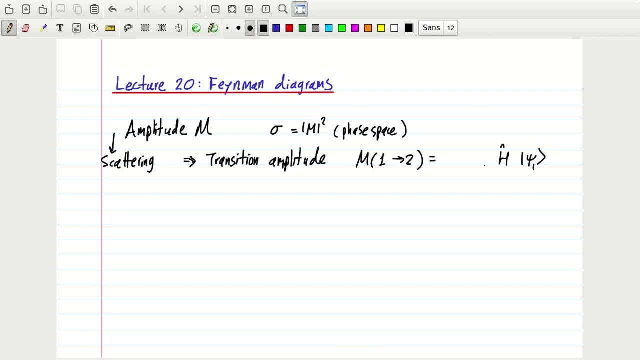 So the Hamiltonian takes you from one time step to the next. let's say So after you've evolved your system with time. then you can see well what is the overlap of this evolved state, Psi1, with a new state, Psi2.. 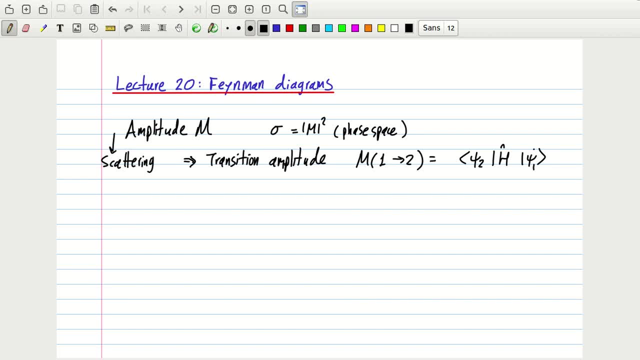 And this is not going to be necessarily 1, because it doesn't mean that H or Psi1 is equal to Psi2.. It's some linear combination of many states and you want to see how much of that is in Psi2.. Now, admittedly, we didn't go into all the details of this. like to fully get the framework that we're discussing here. 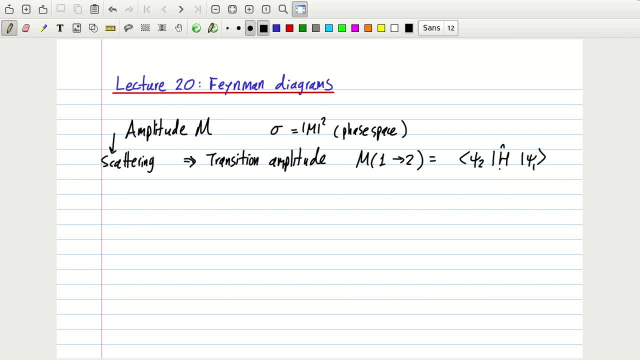 You might want to look briefly into the chapter on first-order perturbation theory In Griffiths. that's where this kind of formalism is really developed. But I think that the main idea should be clear. You can act with Hamiltonian which think of as a matrix acts on some state. 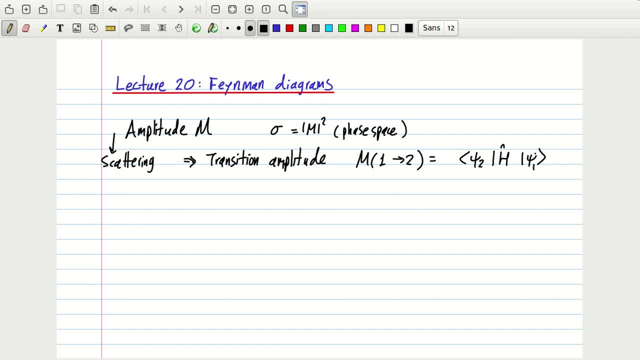 It's going to give you a lot of, I mean some mixed mix of states And this Psi2 on that is going to give you this coefficient c that we were discussing, cn maybe- which if you square it, you get the probability of finding that state, Psi2.. 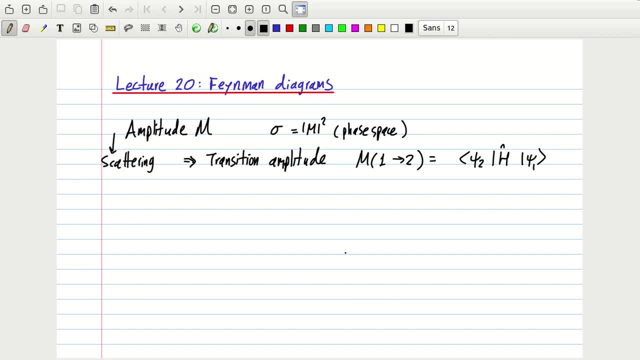 Thank you. Okay, so that's roughly how the regression amplitude works, And maybe I should phrase it: This is probability. This gives us the or m squared gives you probability that Psi1 evolves under the Hamiltonian and is measured As Psi2 at a later time. 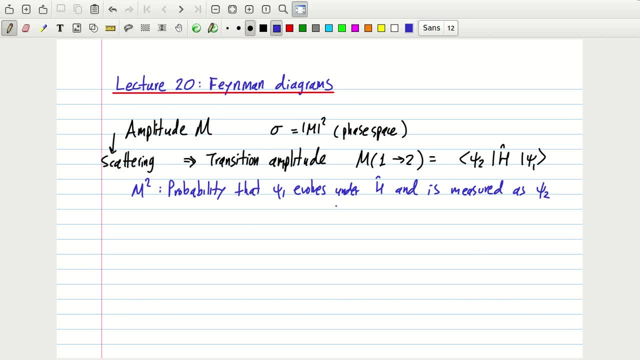 Okay, it starts with Psi1. But it won't stay Psi1 because the Hamiltonian makes it move around And eventually it will be a sum of states, And so maybe you could say: after the evolution we get a sum n, cn, Psi, n. 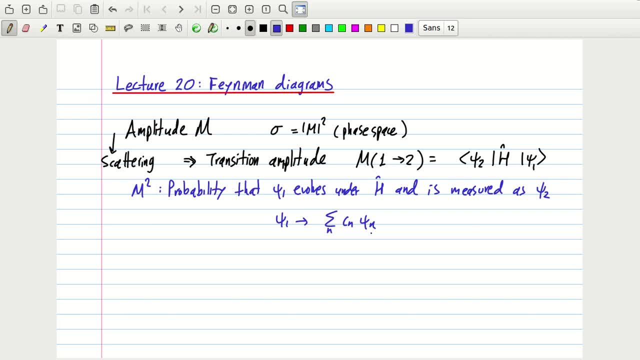 And one of these states is going to be Psi2.. So what we care about is the overlap between This final. so this is now h on Psi1.. Right, that's a sum of these states, And what we care about is specifically the coefficient c2.. 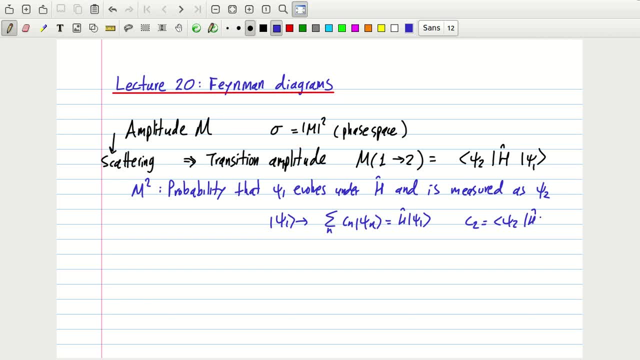 And c2 is the overlap of Psi2, h, Psi1.. Okay, that's roughly what we're doing Now in this case. of course we don't want just our initial wave function. It doesn't describe, just say, an electron in a particular state of some oscillator or something. 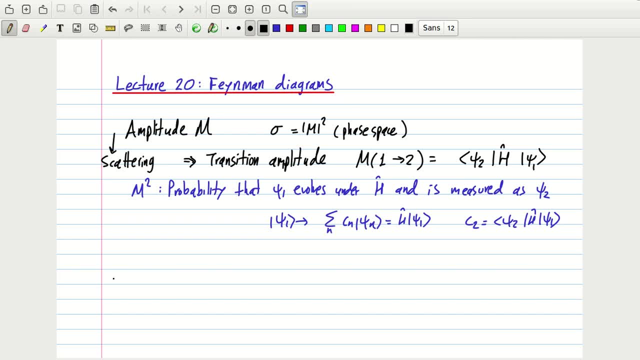 It's going to describe particles, So our initial wave function. So now let's go to the particle physics context, And our initial wave function is going to be something which tells us to have a particle 1, which has momentum, P1.. That's, for now, the information that we need about this particle. 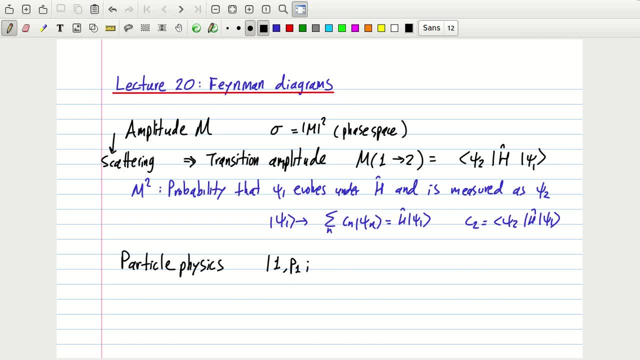 We might need to include other kinds of information in more complicated theories, but we'll stay very simple for now. And then you have another particle 2 with momentum P2.. Okay, so that's our initial state. And then we also want to write a wave function with particle 3, with momentum 3, P3,. 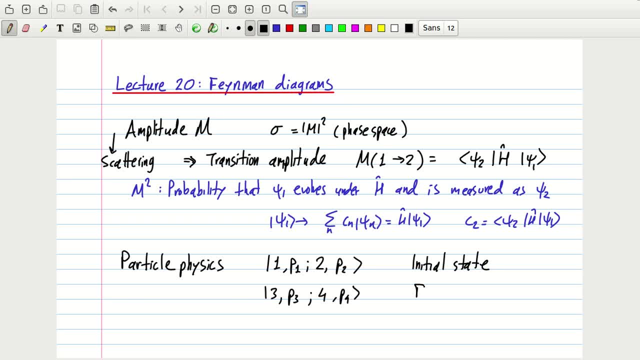 and particle 4, momentum P4, which we're going to call the final state. And now, if you have this and you've specified all your momentum- P1, P2,, P3,, P4, then you can write down the amplitude. 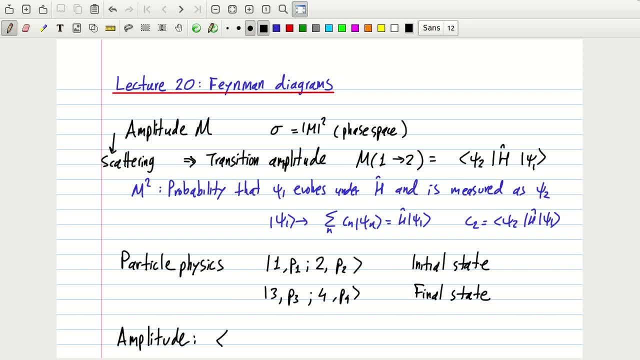 what we're going to call the amplitude, which is the overlap of these states. Simple as that. So 4, P4, with 1, 1, P1,, 2, P2.. Okay, Now, if you calculate this, then if you now take M squared, 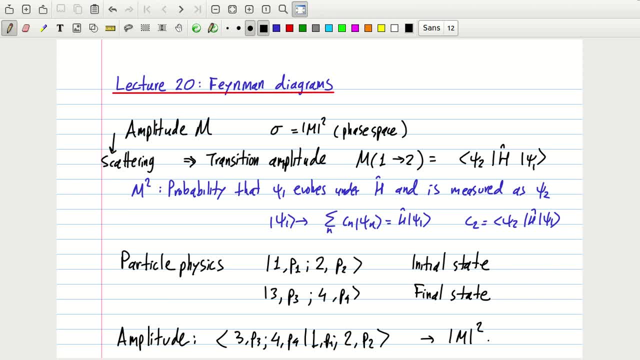 that's going to be related to the probability of finding the specific final state. given this initial state- And sorry, I think I messed up a little bit here- Obviously this not much is happening in what I wrote here. You need to also include, of course, a Hamiltonian right. 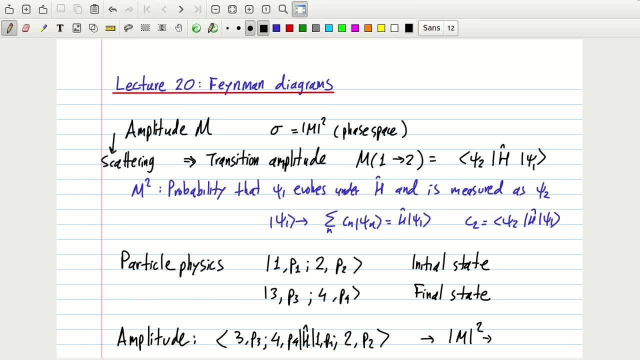 Because otherwise the system is not evolving. If there is no Hamiltonian here, the system is just staying that state. So you're only going to get a non-zero overlap if your 3 and 4 are equal to 1 and 2.. 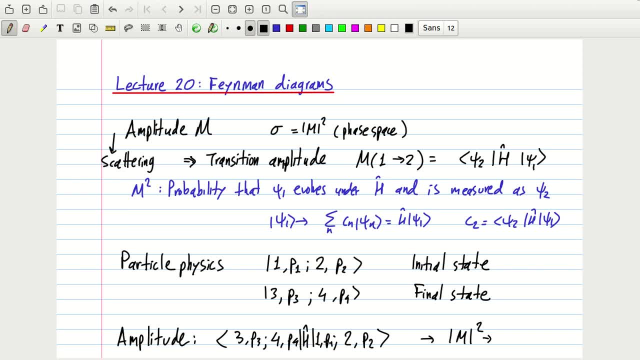 We're assuming orthonormal states here, So the state- let me actually write this by orthonormality you would get something like, for instance, 1 or i P. i overlap with j P. j is something like delta, i j right. 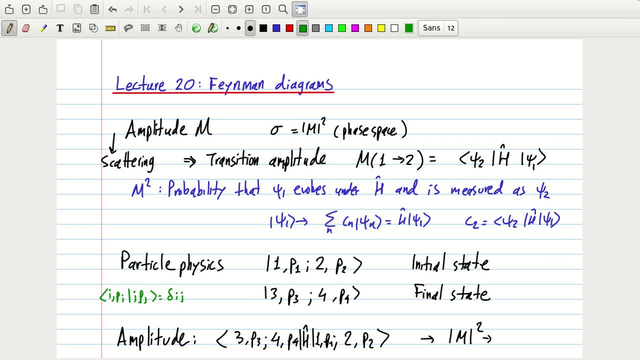 So if the moments are different, the overlap is 0. So that's so, if you started off with 1, 2, and you did the overlap with 3, 4,, you would get a delta function, some combination of delta functions. 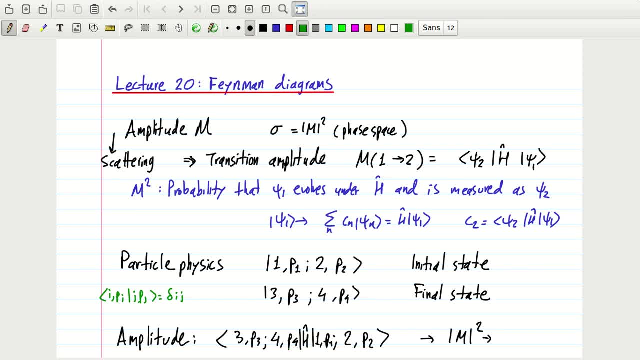 like delta function of 1 and 3, and 2 and 4, and so on. But now we're acting with a Hamiltonian here. that's important. so this state is going to be changing and there can be a non-zero overlap with a different final state. 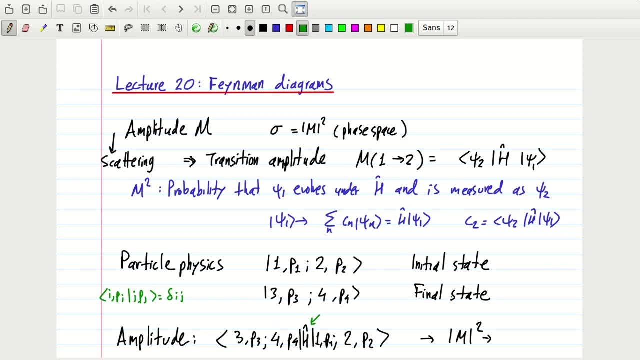 which is not the same as the initial one, And that is going to give us now this M squared, is going to give us the cross-section we're looking for now. of course, now to do this correctly, I would have to go into all the details of the Hamiltonian. 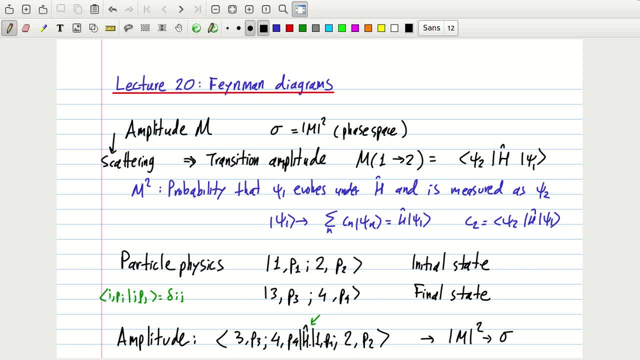 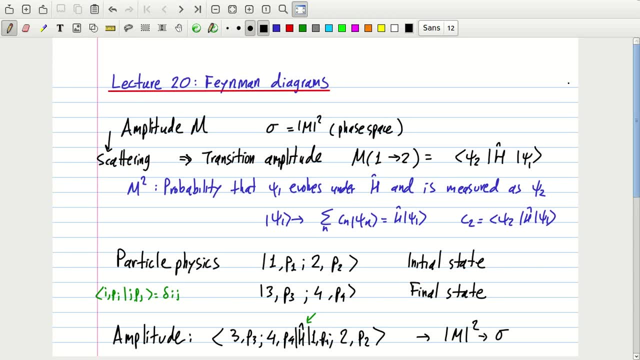 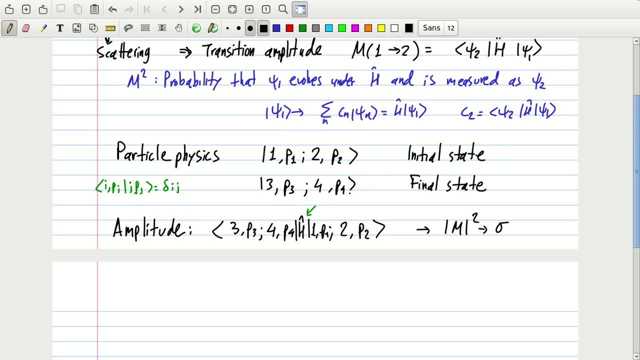 that we have and explain how a Hamiltonian can act on this initial state and evolve it to the final state. Now, this is something that we do in quantum field theory, because to actually do this correctly, there is a lot of background information that one needs to know. 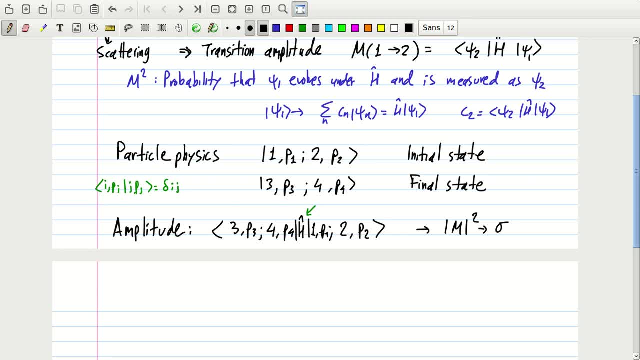 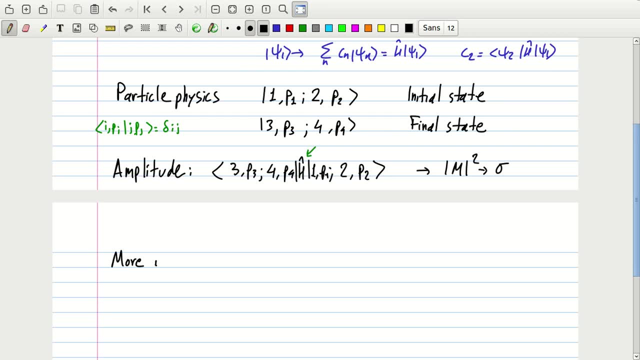 for instance, one should think of these particles as excitations of a field, So formally or somehow more precisely. more precisely say: these states i, pi are excitations of a quantum field. When I say excitations, it's more or less. 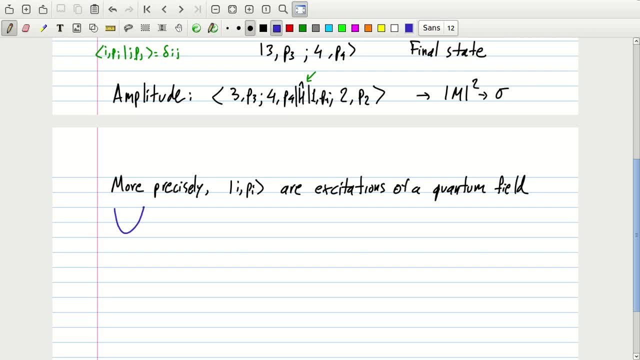 almost exactly the same as what we do in the harmonic oscillator, where you say you have a ground state and you want to jump to the first excited state, and you do that by taking a plus on zero. So that's what we call an excitation. 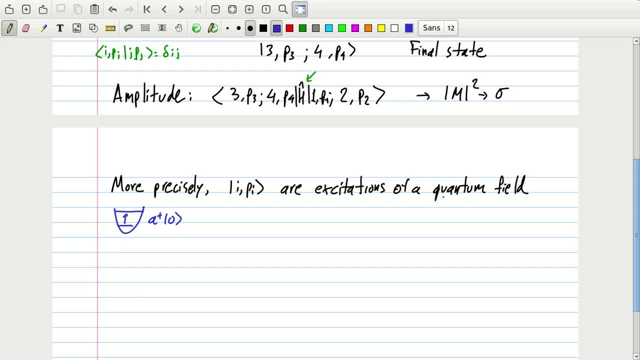 So there will be something very similar, which starts from a quantum field which is in the ground state, which we would call zero, and excites it, and using some oscillators like these ones, like these raising and lowering operators. So you need raising. 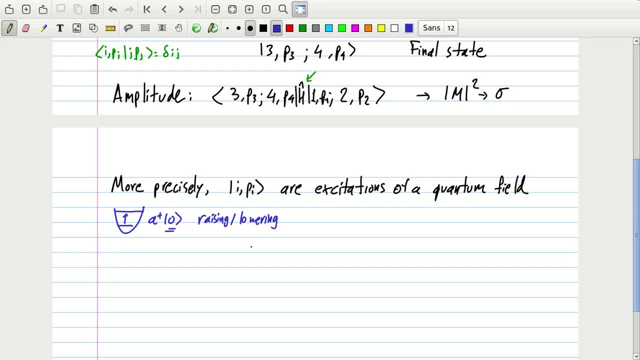 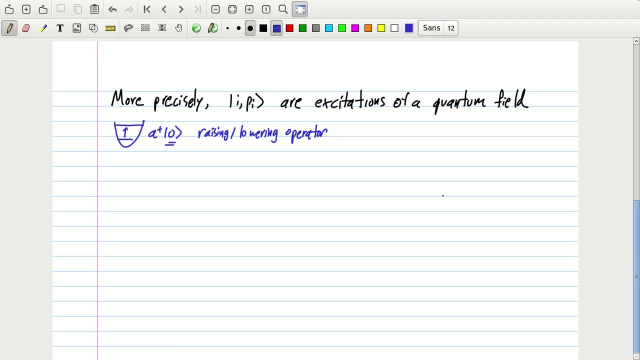 and perhaps lowering, in some cases, operators to actually get these states, the initial and the final state. Now, we're not going to do that because it involves a lot of. I mean, it's not very difficult, but it involves a lot of setting up the framework. 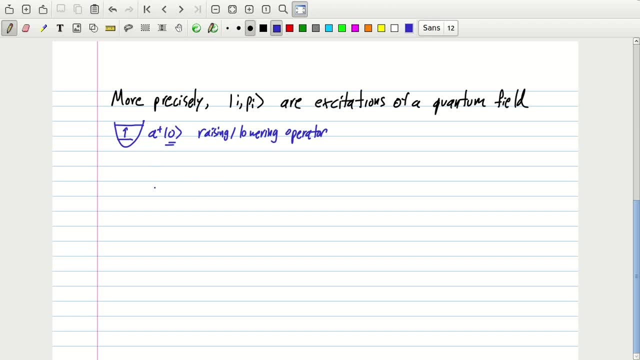 and working on it. It's just quantum mechanics, but it just needs a little bit more work. So we're going to avoid the details in this course due to lack of time, and we're going to just give you a shortcut developed by Feynman. 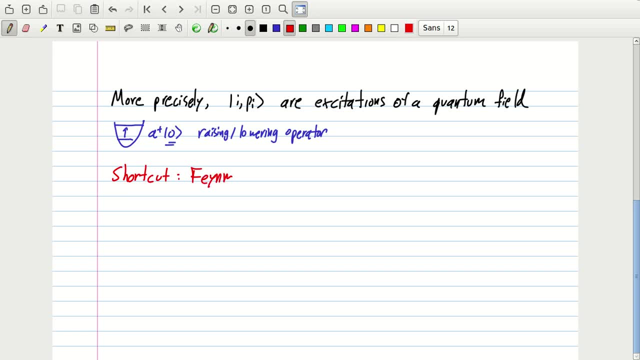 which is known as the Feynman rule. And the Feynman rules are for a given theory. so, given a theory, these are diagrammatic rules for computing the amplitude for a given process, So it's process dependent. 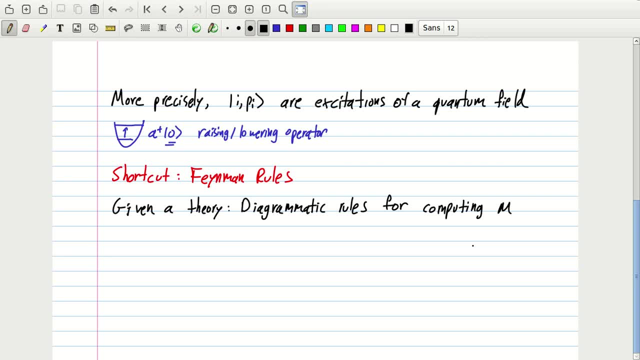 of course. so there's different amplitudes depending on different processes, So you can actually forget everything about Hamiltonians and all that. and if I just give you a set of the rules that Feynman has developed for a given theory, 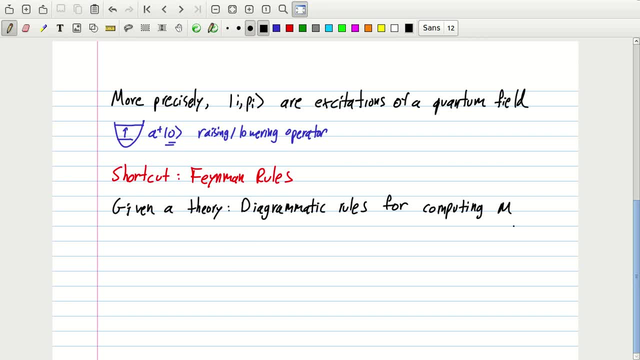 then you can immediately start computing the amplitude for a particular process. Now, because we're also not really interested in getting this in detail, I just plan to give you an overview of how it works. we're going to work in a simplified model. 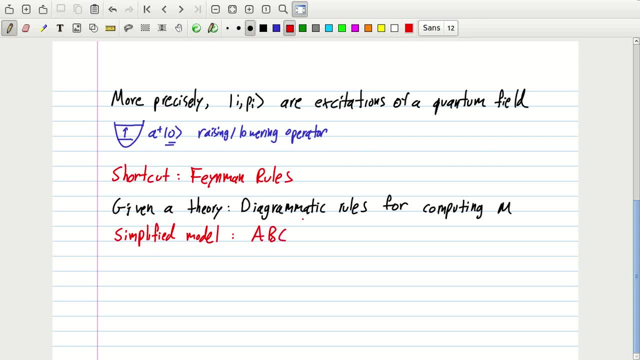 which Griffiths calls ABC. so that's in the Griffiths Particle Physics. so if you want to read more about it, so the elementary particle physics books of Griffiths you can read more about what is happening in this model. but I'll just give you the basics. 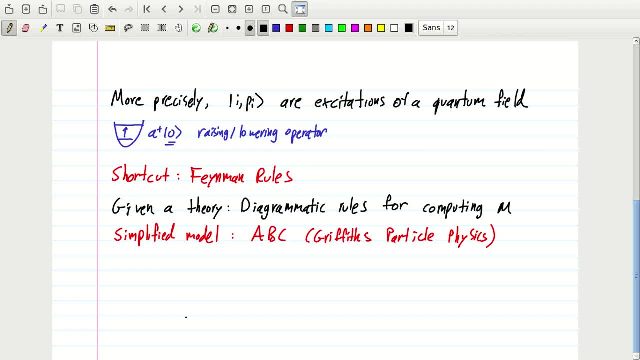 So, instead of doing something complicated, with quarks and photons interacting, which can get a little bit tricky, the problem is that basically, what we want is we want to ignore spin, because that complicates the Feynman rules. 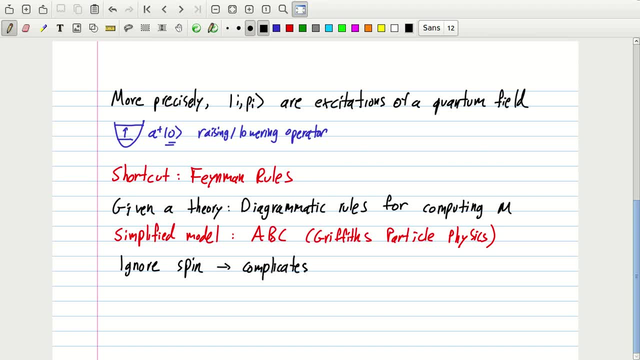 Because you always have to make sure that spin is conserved and you have to worry about combinations of spin that match and all that, and because in QED, for instance- so in QED, you have electrons which have spin. 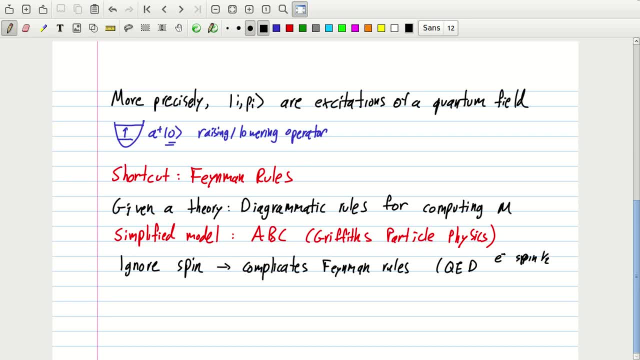 spin half and they're also charged plus minus. so you have electrons, positrons, and you also have gammas, which have spin one. now, gammas are also kind of complicated. photons are complicated in the Feynman rules. 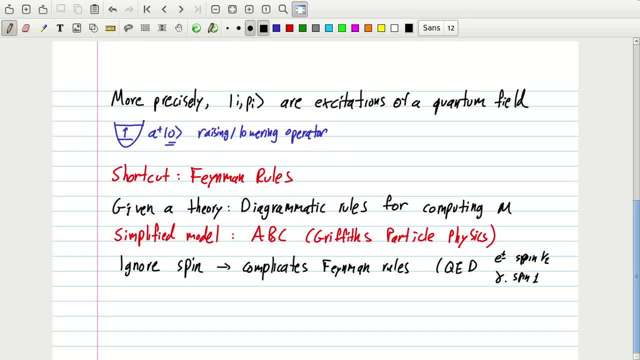 because they have some property called gauge invariance, which means that not every component of the photon is physical. so when I say physical, I mean that it actually is a measurable degree of freedom. they have some degrees of freedom. so remember, a photon is spin one. 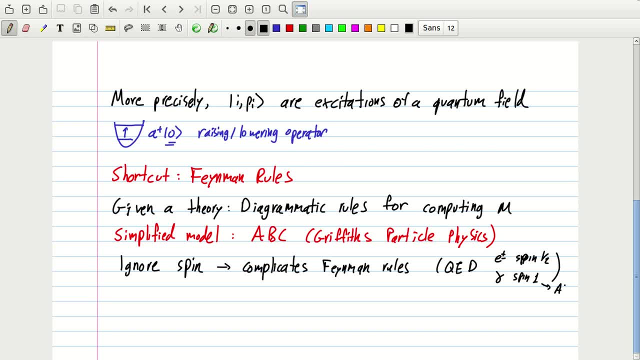 and that we describe in four dimensions as a vector, a mu. but a photon doesn't have four components. it actually only has two, which are the two different polarizations. so two of the components of the photon are not relevant for physics. 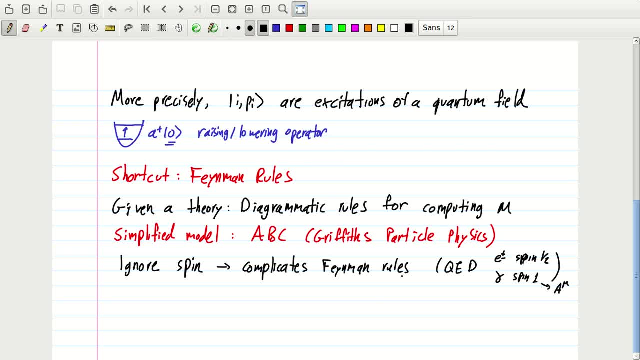 and the Feynman rules need to kind of take that into account, and that complicates things quite a lot. so instead we will work with scalars, and even though this is not very realistic, because in the standard model there are no real scalars- 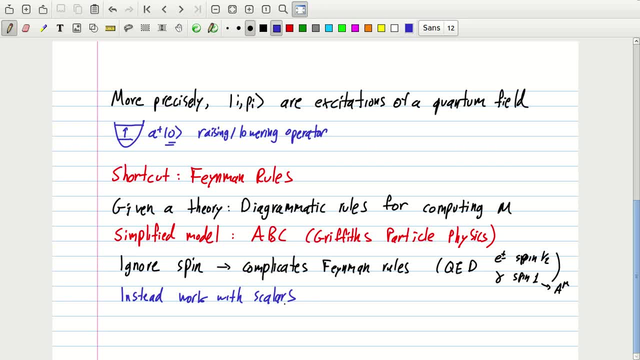 I mean there's only the Higgs particle, and even the Higgs particle is not exactly a neutral scalar. it interacts with the other particles, so it's not something that is very realistic for the standard model, but at least it gives you an idea of. 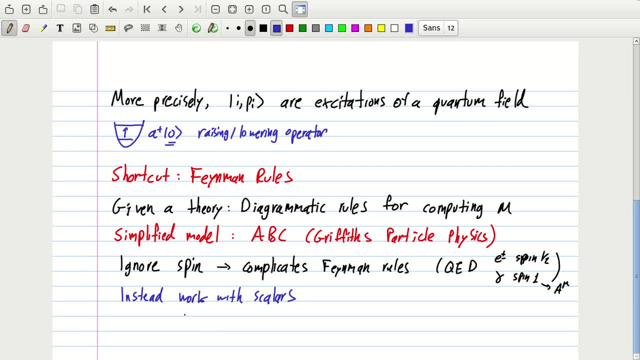 in a clean setting of how the Feynman rules work. So we will have three scalars, just to make it not too trivial. so three different scalar fields- A, B and C- and they're going to have different masses. 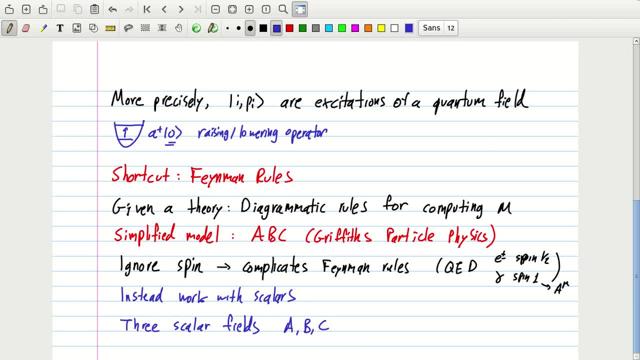 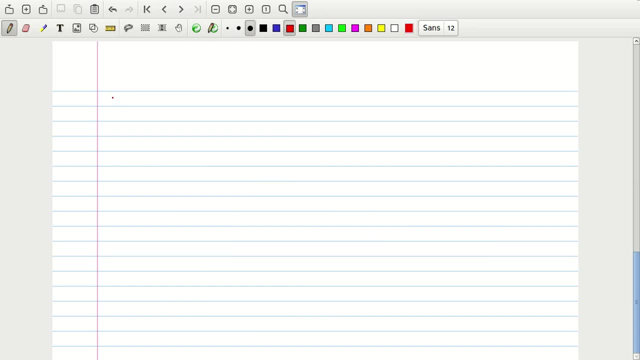 we're not going to worry too much about the mass. what we care about is: what is the interaction? so what the Feynman rules tells us is that a field can do two things. so a field can propagate, so a field can go from one place to another. 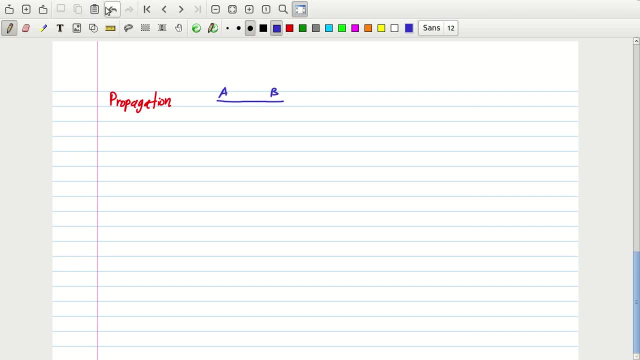 so we can write it like this. sorry, that was wrong. so each of these fields B and C can move from one place to the other like so, or you can have an interaction, and that's the non-trivial part. 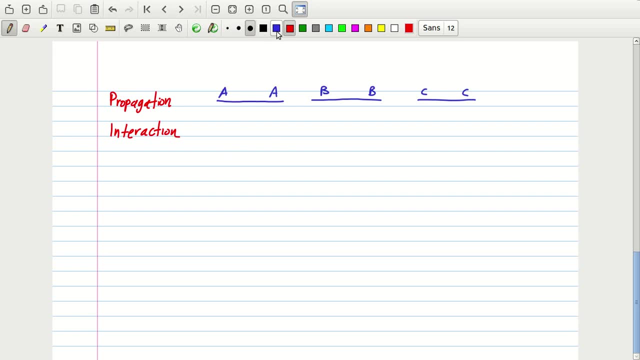 Now, in this theory we're going to assume there's only one interaction, one kind of interaction, and it's going to look like this: so where an A field can decay into a B field and a C field, or a C particle, maybe I should say better. 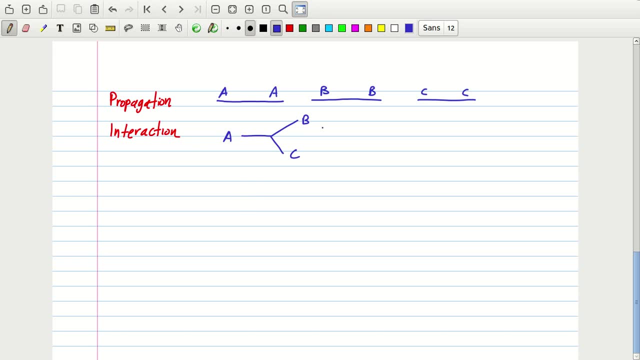 And now in interaction this is called a vertex, and we've seen vertices like this before, when, for instance, a quark decays into a different quark and a W or a Z particle. so this is a simple case of that. 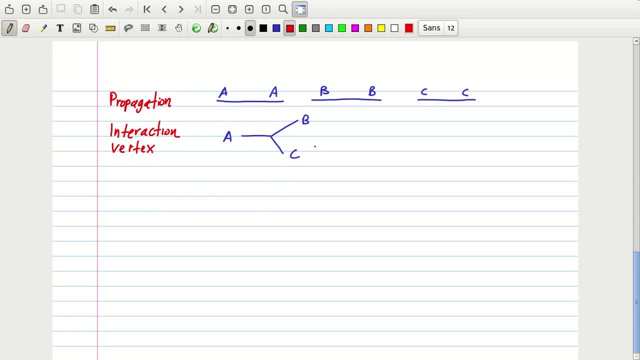 because in that case, although we can easily write it schematically, actually computing what the diagram means would be quite complicated, While in this case there is nothing really special to it. all that you say is that, well, whenever you see something like this, 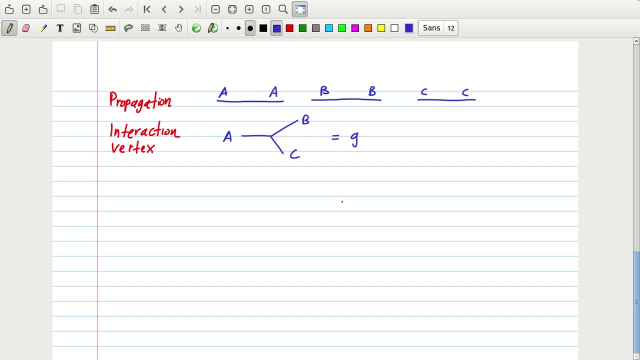 this is equal to a constant, G, known as the coupling constant. Okay, So it tells you how strong the interaction is and, of course, we're going to assume that G is a small constant, and we'll see why, because we want simple diagrams. 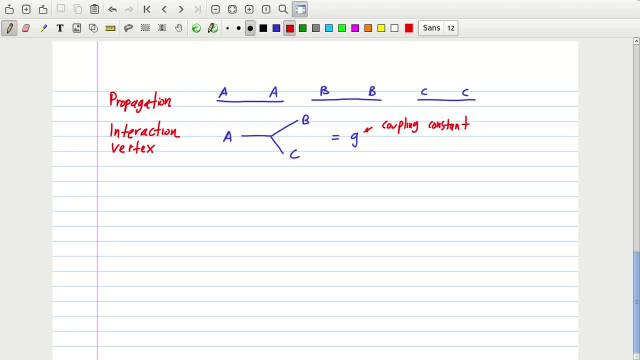 to be bigger than complicated diagrams, and that you can only do if G is a very small number. But you can think of this coupling constant. now, if this was so, this is an analog of the basic QED interaction, which maybe I'll quickly state here. 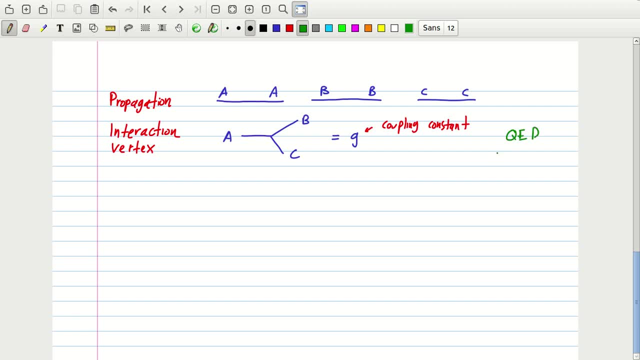 say QED. QED is quantum electrodynamics. there's actually only one interaction, which is that an electron produces a photon. so you can think of A and B as being electrons and gamma being a photon. Okay, there are similar interactions. 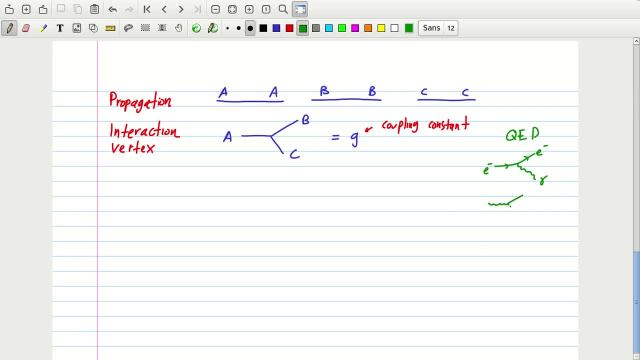 that you've already seen, like a photon giving an E plus, E minus. but these are variations of the same thing, because remember that if you take a photon- sorry, an electron- moving in the opposite direction, it becomes a positron. 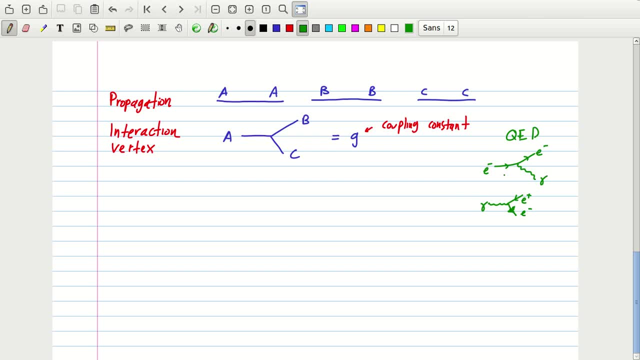 So it's not really a new particle, it's just the antiparticle you can get by just moving the line around Here we don't have any particles or antiparticles, we just have these three scalars and we assume they're neutral. 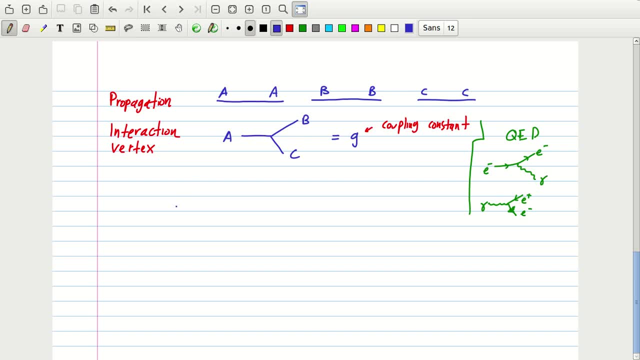 and they're their own antiparticles, we don't need to worry about antiparticles. Okay, so that is basically the interaction. you need to also include the momentum, so you can call this P1,, P2,, P3, because of course, we need to. 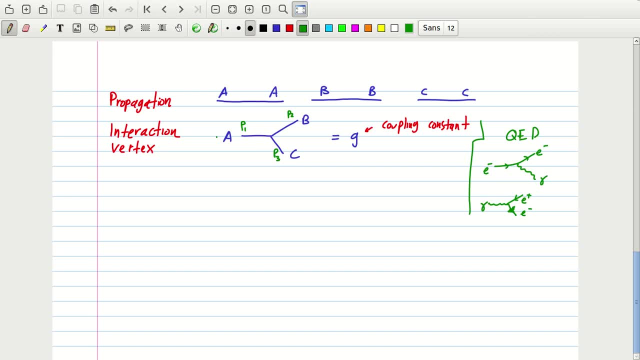 when we put everything together, we need to know whether this, what is, the momentum dependence of the amplitude. So, even though this is the only vertex, every time that you see a Feynman vertex, of course you're allowed to change things around in time. 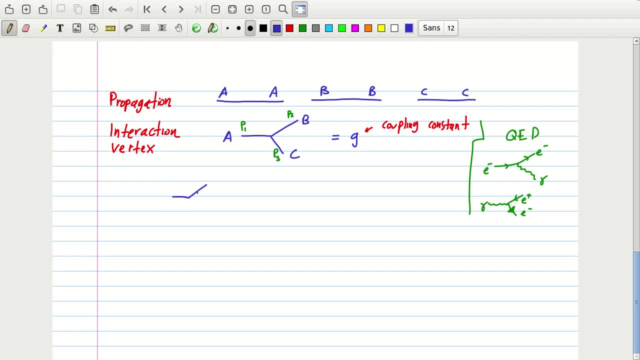 so nobody's stopping you from, instead of A B C, of writing for instance C B A. if A B C is allowed, then C B A is also allowed, or A C, B, and so on. 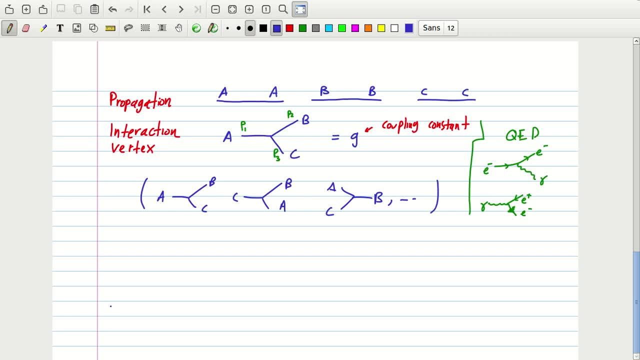 Okay, so you can have all of these vertices, which are the same as this one, if you reverse some of the lines. So now, to start calculating an amplitude, we need to decide first of all which amplitude to consider. So we need to specify. 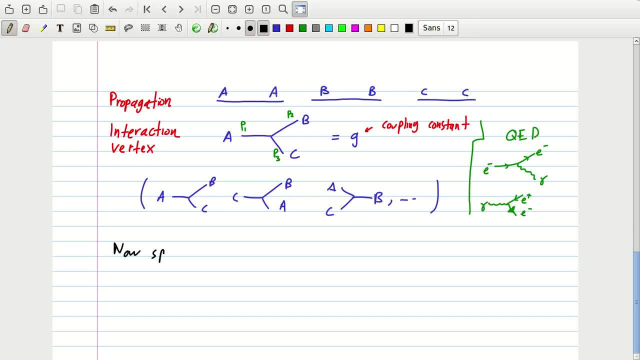 okay. so now we need to specify initial and final states, And we're going to be simple here. we're going to just write something like A B going to A B for now. So we're just going to worry about A B going to A B. 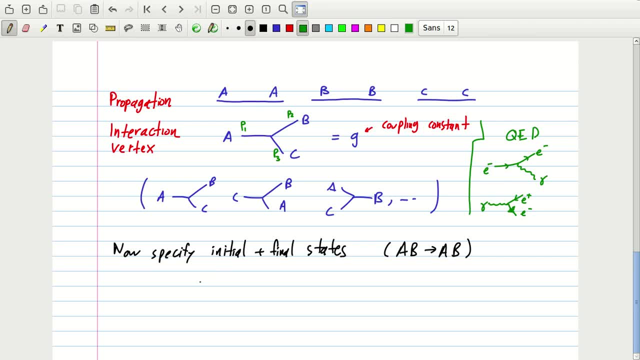 which I can write schematically as so. So I have a particle A with momentum P1, and I have a particle B coming in with a momentum P2.. And what I want out, and I'll write it in this order, just to simplify my life a little bit. 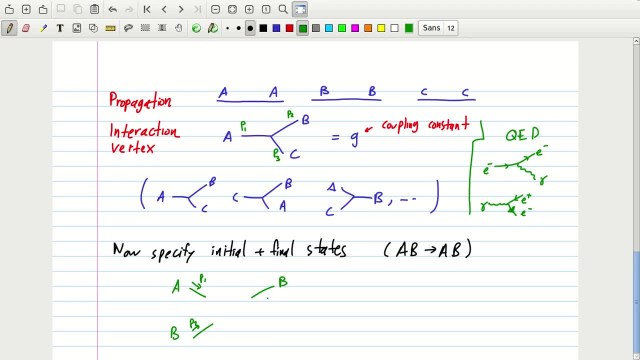 I'll write a particle B coming out like this with a momentum P3, and a particle A coming out with a momentum P4.. Now the question is: by the way, time of course moves to the right right, So that's why I'm calling these the initial state. 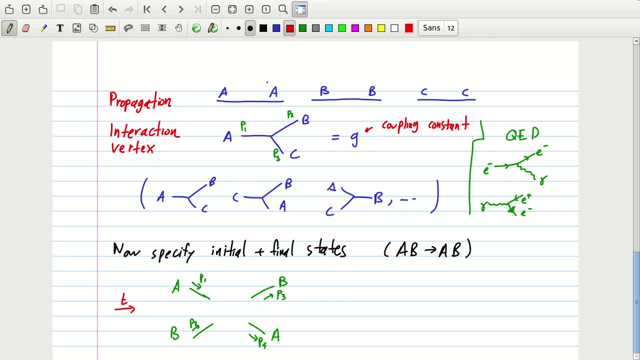 and these I'm calling the final state of the interaction. So the question is: what happens in the middle? So here we often draw a blob which tells you that you need to add. so that's actually the real Feynman technique. 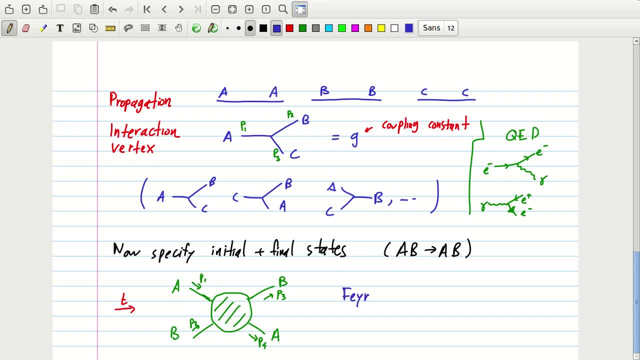 or the Feynman approach, which can be proved, of course, very concretely, but now we're just giving the rules- is to sum over every possible intermediate state or intermediate process. let's say This is not very different from: 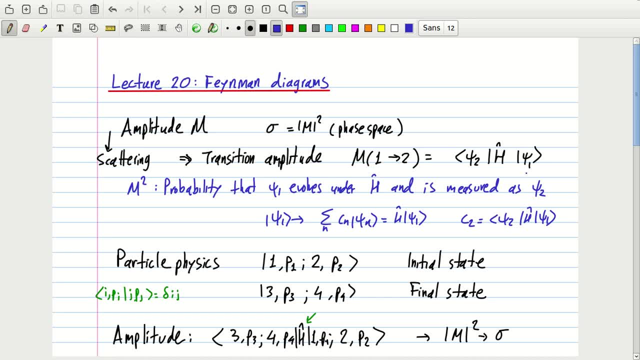 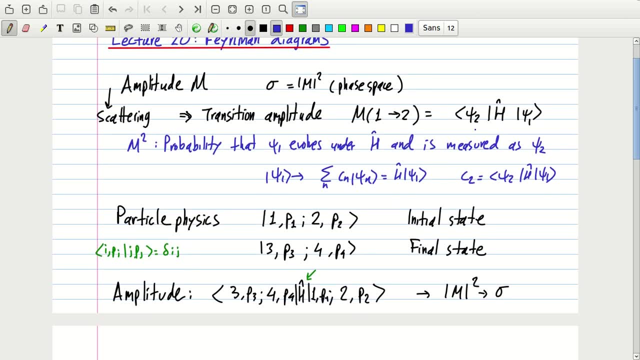 what you would do in standard quantum mechanics. if you have some Hamiltonian that's rotating things around, you would also need to do exactly the same thing To find the overlap you need to do, and we've done some examples of this in quantum mechanics. 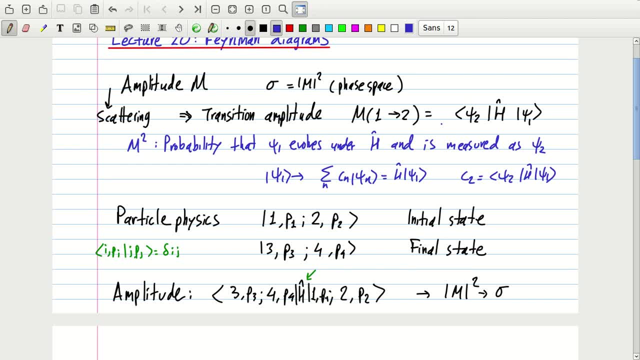 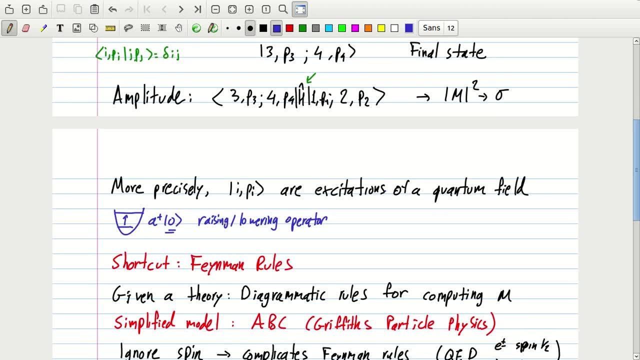 with oscillators, raising and lowering operators, where you need to add all the possibilities. Suppose an energy level first goes up two times and then goes down once, or goes up once, or goes up five times, then goes down four times. all of these will contribute to the amplitude. 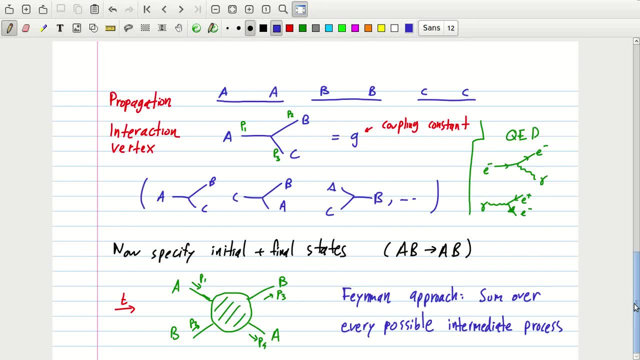 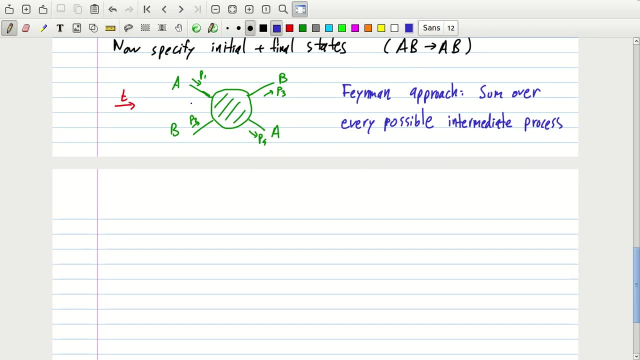 of going from zero to one. So that's exactly what we're doing here. in this approach, we need to find all the possible intermediate steps that take you from AB back to AB- or BA in this case. Now let me emphasize that it doesn't really matter. 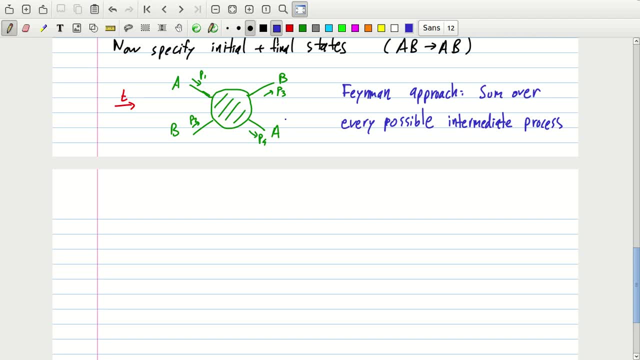 it matters a little bit for aesthetics, but it doesn't really matter at this point whether I write AB or BA here. There are theories where this is important, called planar theories, which things should not cross if you write them on a piece of paper. 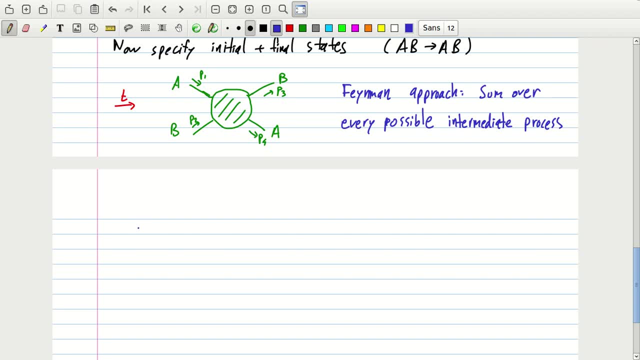 but in our theory we don't worry about that either, but, as you see, it will make it a bit simpler to draw some of the diagrams, Okay, so how can we get now from AB to BA? And this is where now you start needing to become creative. 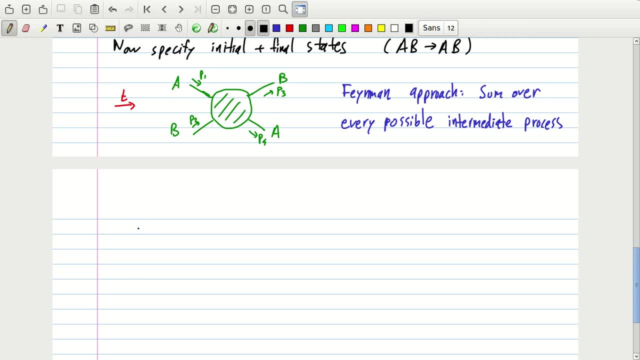 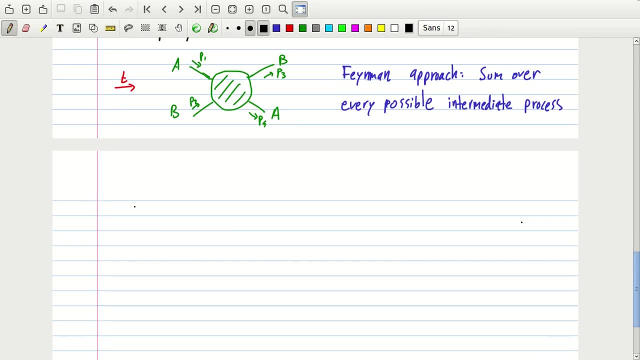 because you need to start looking at combining your vertex, all your vertex that you have, in such a way as to get this transition to happen. So one obvious way to do this is to start with AB, create a C, and now this C is going to 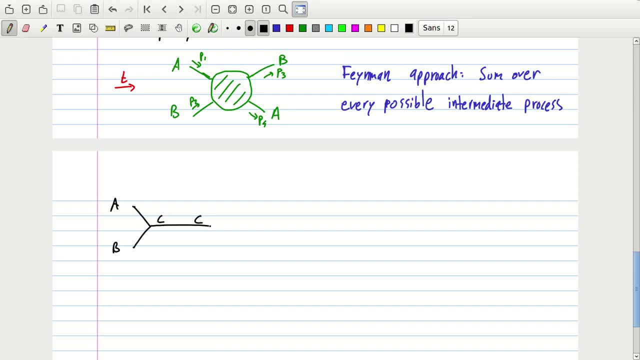 of course propagate using its propagator and eventually it can decay. and when it decays, it can decay to a B and an A, And we need to assign to this C also a momentum which we're going to call Q, which is known as an internal momentum. 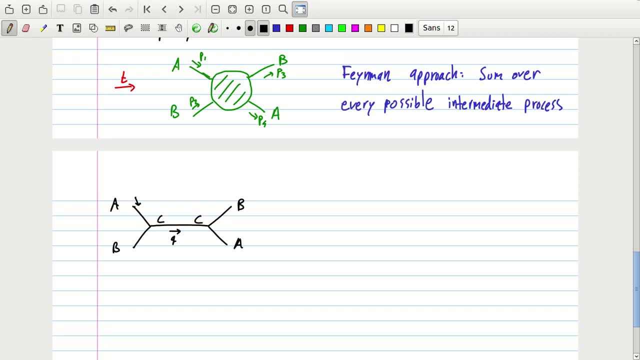 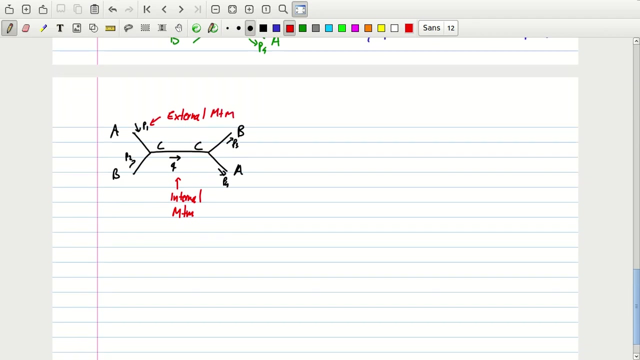 So we still have- I'm not going to keep writing- the external momentum- P1,, P2,, P3, and P4, but you should always remember that there are these external momentum and this is the internal momentum. Okay now, the difference between internal and external is more than just that. 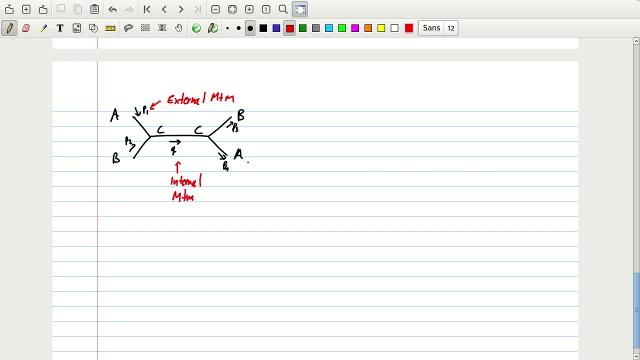 these are the particles of our initial and final states. it's also that we can choose what our external momentum, So in a given process, we can decide: oh okay, we send an A and a B particle scattering with these momenta and we measure a, B and A particle. 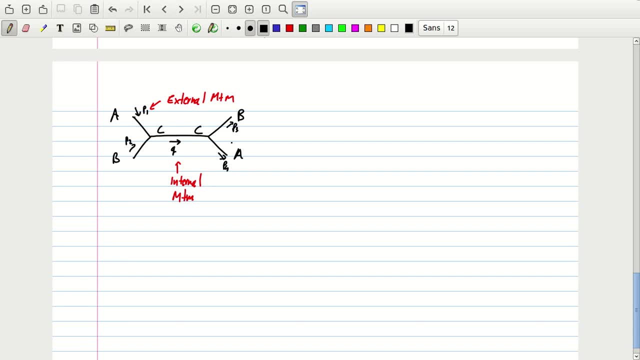 and we can choose which momenta to measure, because we can measure everything, but we can measure the momentum and say, okay, we only care about the transition from A to B to B to A with specific external momentum. So this is something that we can fix. 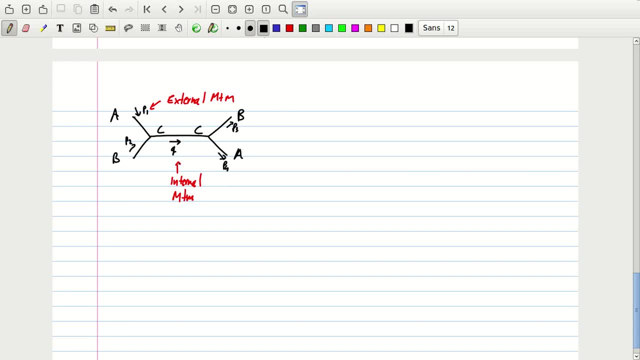 while the internal momentum is something that we cannot actually fix And, as we're going to see, it's part of the rules that we're going to need to integrate over this internal momentum. This is not very different from free and dummy indices. Free indices are an equation you can fix for yourself. 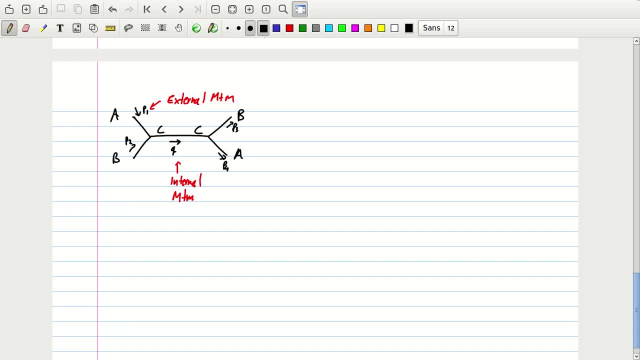 dummy: indices: you sum over. In this case, instead of indices, we have momentum, which are real numbers, so instead of summing, we take integrals. We're not going to go through this in any serious detail at this point. Okay, so this is one diagram. 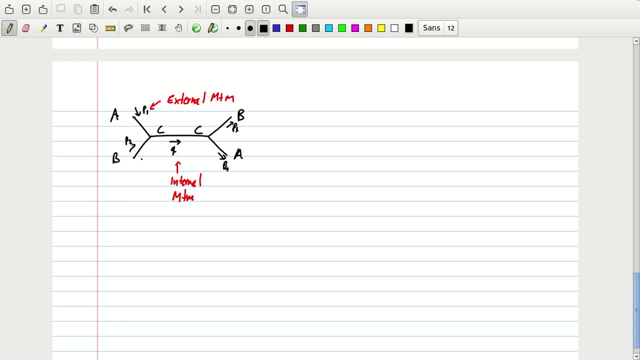 but, as you can imagine, there's actually more than one possibility of doing this, and another obvious possibility of having this process happen is, instead of A and B first meeting up at the vertex here, then creating a C, and then that C decays. 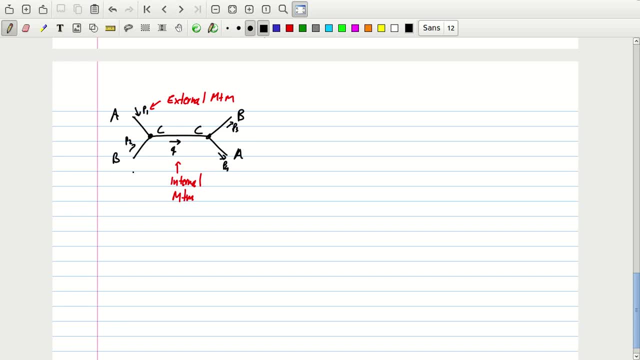 what could actually happen is that this A and this B could meet up first, So you could write something like a B meeting up giving you a C, which then meets up with this B and this A, And this is an equally valid diagram to the original one. 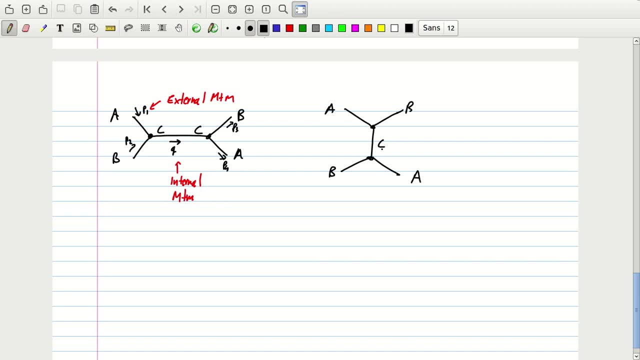 Okay, so now you can try to check: are there any more? And you won't find any really different ones. Of course, you can write this in slightly different ways, but what we care about is the graph, the topology of the graph. 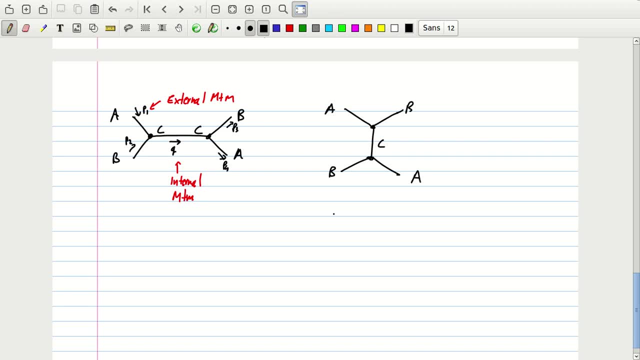 and how many are actually different. how many different graphs do we have that provide this transition? Okay, so when I say C, maybe I should be a bit more clear. What I really mean is you create a C which propagates and gives you a C. 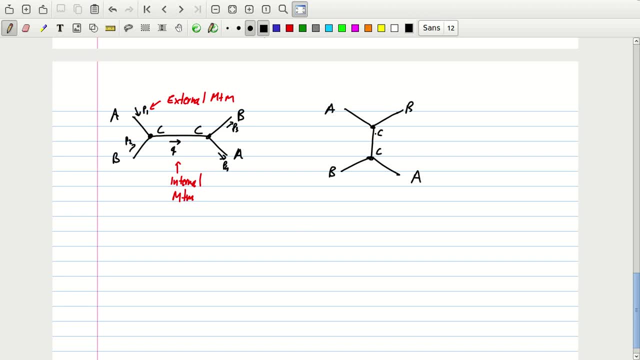 Now, because these lines always are, say, C or A or B, I often will write it in the middle instead, just to avoid writing the thing twice. But I think it will be clear what I mean, And here there's also going to be a momentum. 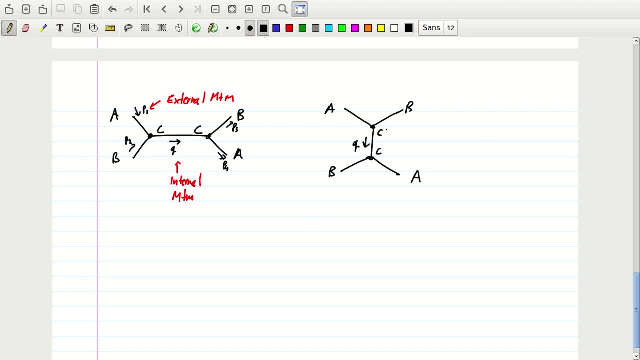 Q. but as you're going to see when we explore these diagrams a bit better, a bit more in the following, the relation of this momentum Q to your initial momenta is very different in these two diagrams. because, you see, now P1 is here. 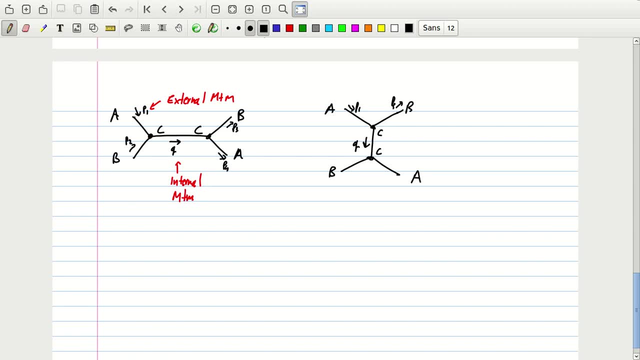 P3 is here and these are the diagrams that actually arise in this vertex with C. Well, here you have a P2 and a P4, and now P2 and P4 talk to this Q. Well, here, actually it's P1 and P2 that talk to Q in this vertex. 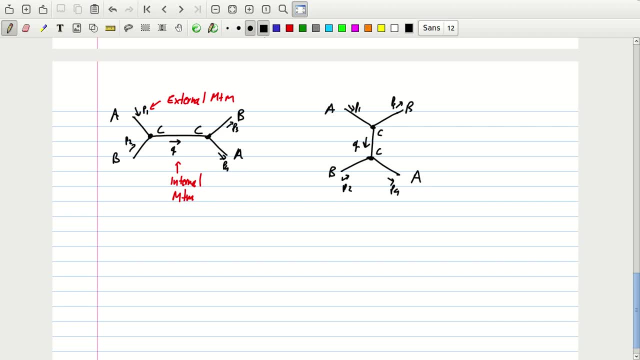 and it's P3 and P4 that talk to Q in this vertex, And we'll see that that actually makes a difference. maybe not so much in this specific simple example of scalars, but in practice this makes a very big difference between these two diagrams. 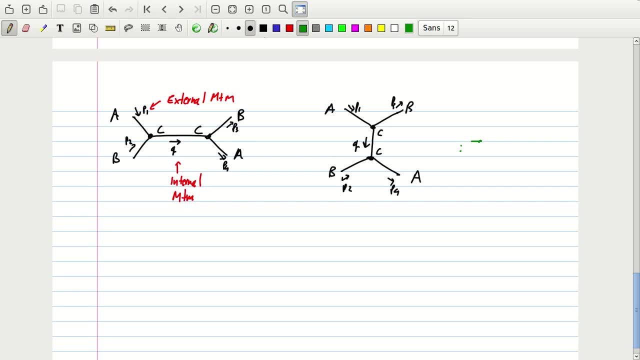 Now these are known as tree-level because, well, I guess they look like sticks or branches of trees, and if you write more complicated ones, it'll be clear. I mean, you can write depending on how many external particles you have. 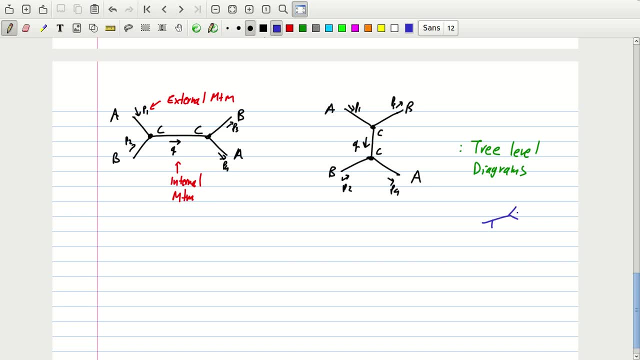 you can have particles with various which start looking a little bit like trees, But these are of course. these are particles with many more external states. This has eight external particles in this case. We're only focusing on four for now, But the point is that we're not done. 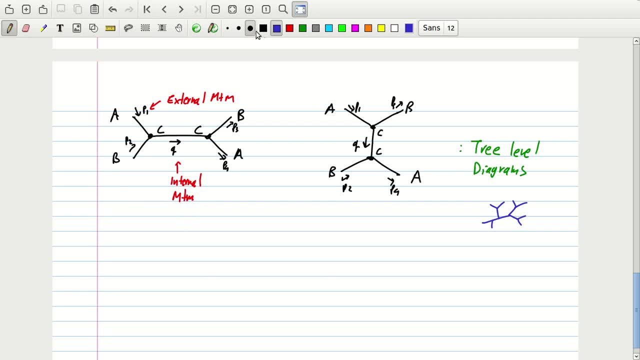 because there's more processes that can happen, which involve your intermediate state also doing something before it reaches the final state And, for instance, what can happen is that your A and a B can create a C, but that C can split into an A and a B. 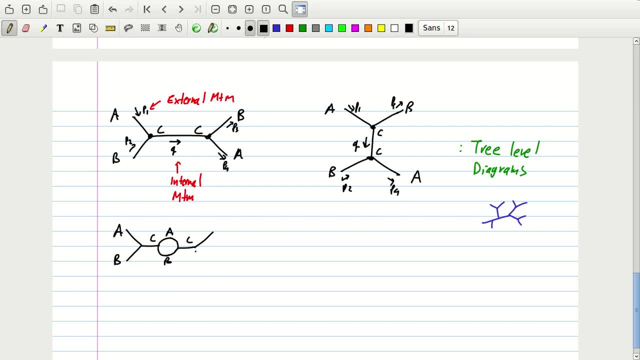 which also then meet up again, create a C and give you the B and the A. Okay, So that's another valid diagram, But of course it's not necessarily the end of the story. You can also have diagrams that are variations of this. 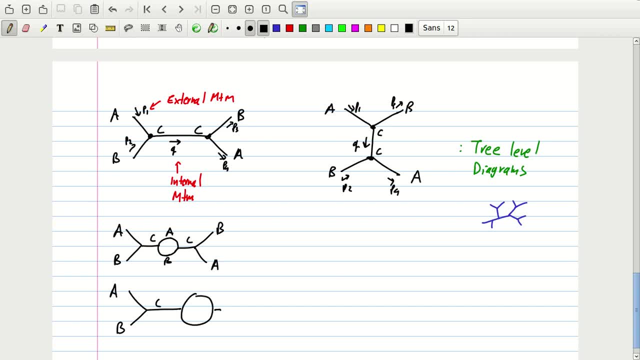 where, for instance, your C? let me write it a little bit bigger to illustrate what I want to say, So you can have this: and here this is an A, this is a B, so nothing stops this A from creating a C. 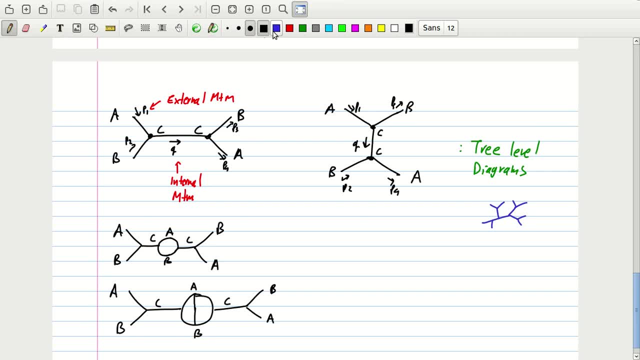 Sorry, maybe I should write it a little bit better. You can have a vertex where this A becomes a B, emitting a C, and this now B becomes an A. This is also allowed because, as you can see, I mean the only rule is that at each vertex. 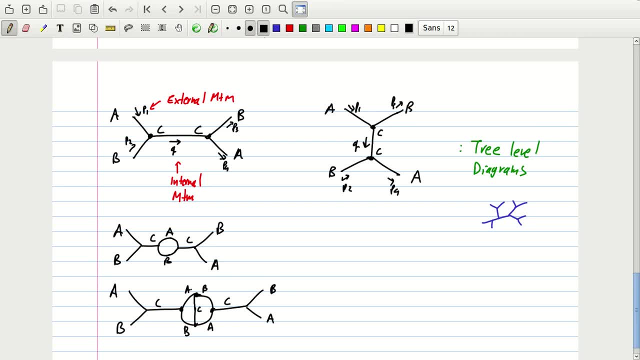 you have to have ABC, And this is always. this is true in this case, Of course. if I had written something else, if I had tried to put C here, it didn't work because there is no vertex between C- C. 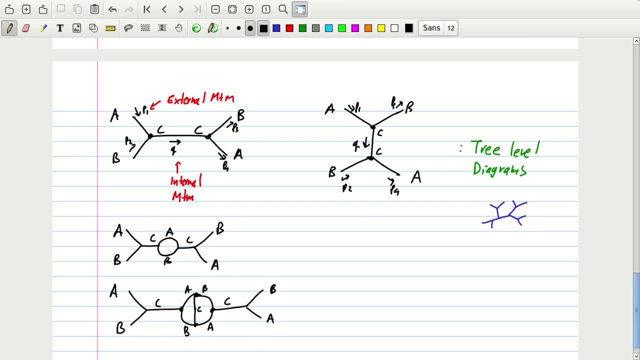 and A, for instance. But if you can manage to write something like this, then this is also fine, And you can have many more of these kinds of diagrams. For instance, I can write something like this: A, B, A, B. 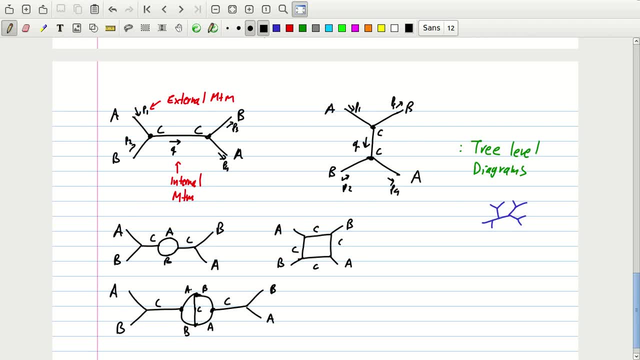 where these are all Cs. That's also no, that's actually not going to work. Let's see, If I put a C here, let's see No, because you see that the problem is, if I do this, I'm going to get a C C here. 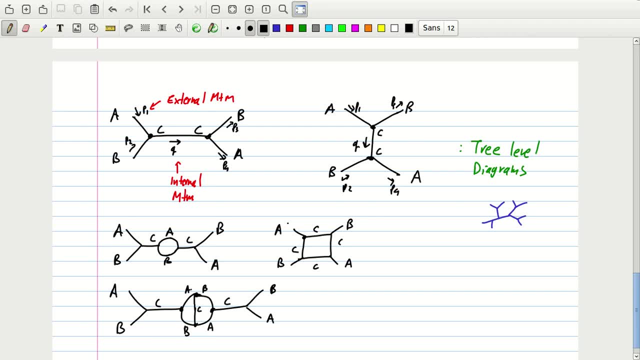 and that's not something that I want. So actually, no, this is not allowed. It would probably only be allowed if I were to split it in some smart way, so that this becomes actually a A, B and this becomes a C. 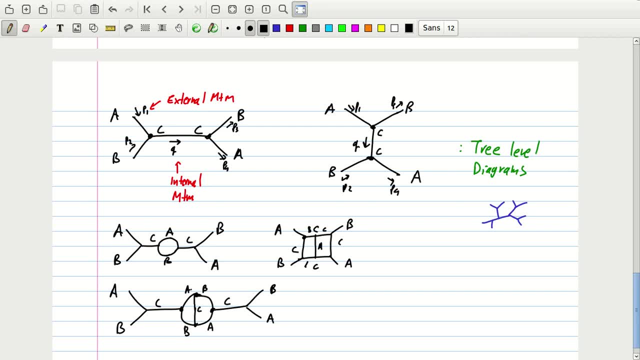 and this becomes an A, So you can start thinking about the different kinds of cases you can have. Actually, I don't see, maybe this actually does not work, So maybe I was a bit too fast, But you can try it and you can see what might happen. 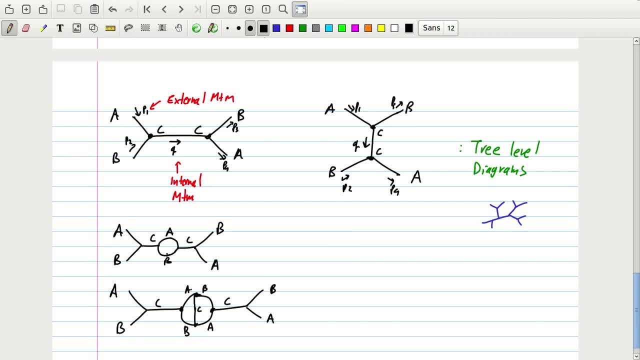 But you see what the problem is. If you start to try to write a diagram, you'll run into problems, that you have the same vertex appearing many times, What is also possible to happen. let's see, These are definitely allowed. I'm trying to see if there's anything more. 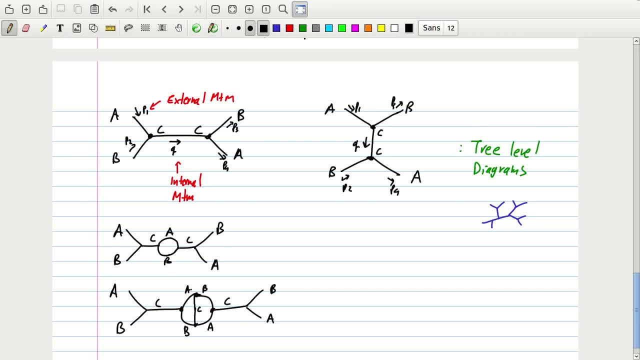 that I can get at this level. But okay, that's actually an exercise for you to try to implement. And there definitely are many more of these diagrams and we'll discuss a few in the tutorial perhaps, But the point is, these are called one-loop diagrams. 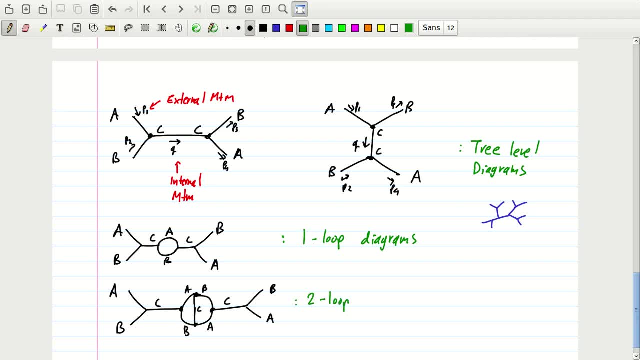 These are called two-loop diagrams, based on, as you imagine, how many loops there are in the diagram. Okay, So, something like this. So, Okay, so I hope it's clear. By the way, if you had, Okay, I'll write in the next slide. 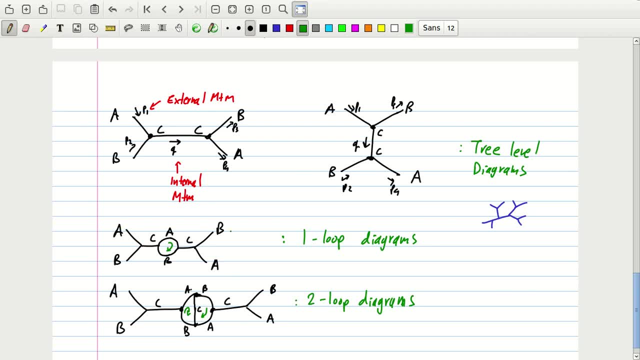 But if you had a different process, for instance cc giving you cc, then you could have that diagram that I wrote earlier, But maybe it won't appear in this specific process, And now you can go on and you can write n-loop diagrams. 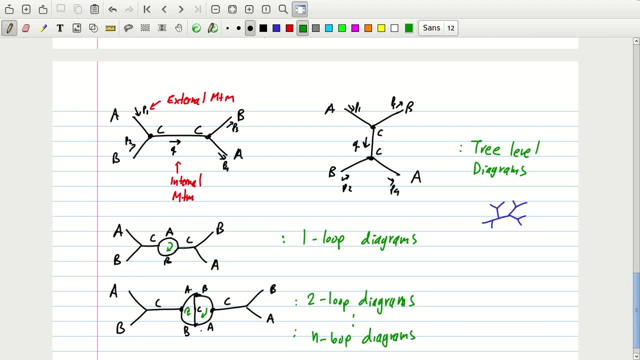 Right. So you can get as complicated as you like with this, because you can keep adding lines. You can add a line from here to here, for instance, and that will change some of the things, but it will be allowed. So from this part to this part. 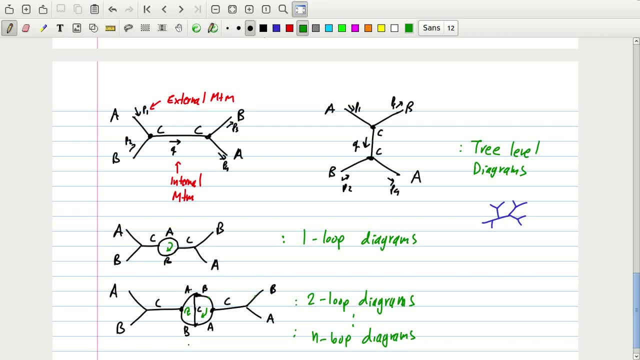 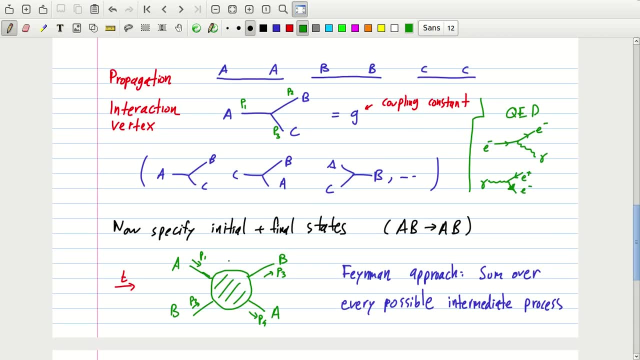 if you take care of all the c's and b's, it will work, and so on. So basically, you get infinitely many diagrams. So that blob that we had here actually stands for infinitely many diagrams. So what is the logic of organizing these diagrams? 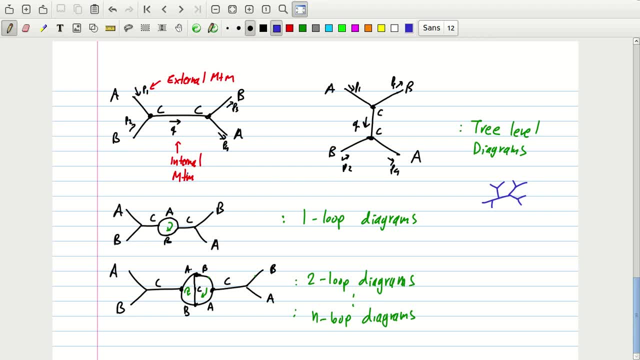 Well, it's what I said before, that if you look at this three-level diagram and you look at what is the order in this coupling constant g, what you'll find is that there's a g here and a g here and the same here. 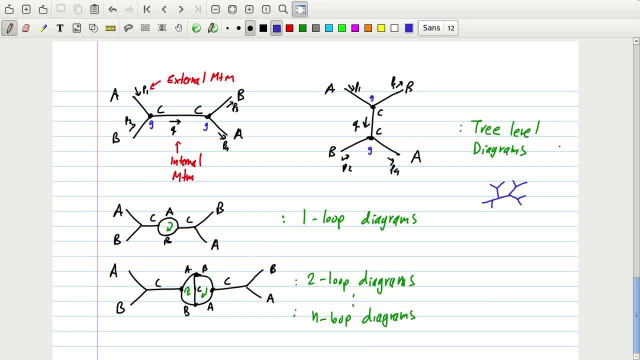 There's a g here and there's a g here. So three-level diagrams are of order, g squared. So if you multiply, Basically, the rule is you're going to have to multiply the factors of g and you get g squared. So three-level diagrams for this process. 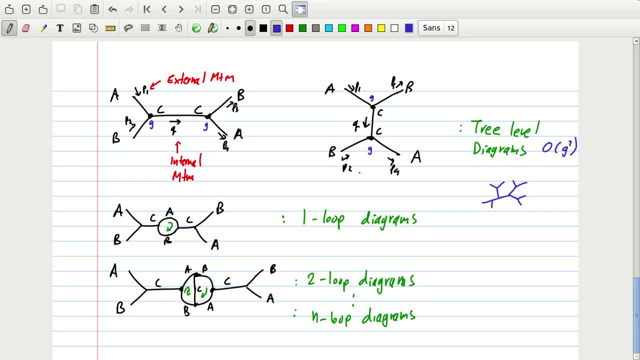 which is four particles total. two in, two out are ordered g squared. If you had five or eight, it'd be different. I mean, you can calculate here. This is three-level, but how many vertices are there? One, two, three, four, five, six. 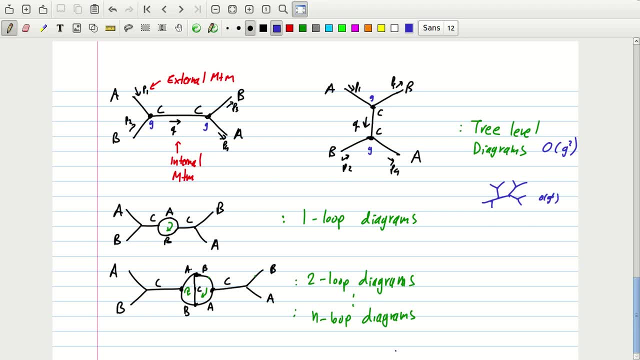 So there should be order of g to the sixth, for instance. So it depends on how many particles you have, But for four particles this is order g squared. but now if you look here, there's a g, there's a g. 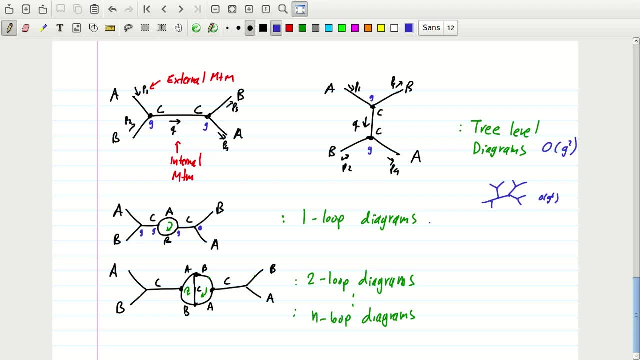 there's a g and a g, so the one-loop diagram is order g to the fourth. The two-loop diagram you can check is one, two, three, four, five, six is order g to the sixth And that continues like that. 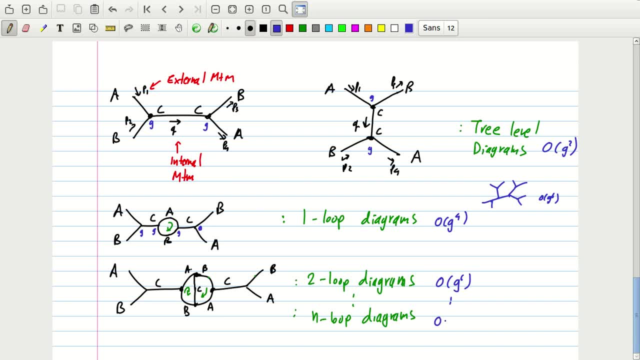 so for n loops you're going to get something like order, order of something like g to the two plus two n, if I'm not mistaken. So at one loop it works, at two loops it works Okay. so I think it works. 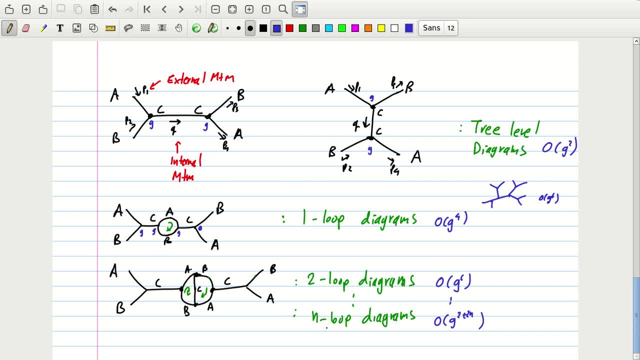 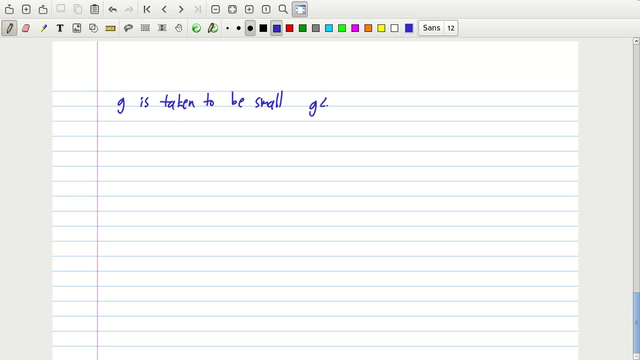 So the point is, even though you have infinitely many diagrams that you need to include, they have different values of g, And if g is small, g is taken to be small, which means that you can ignore higher loop diagrams, depending. 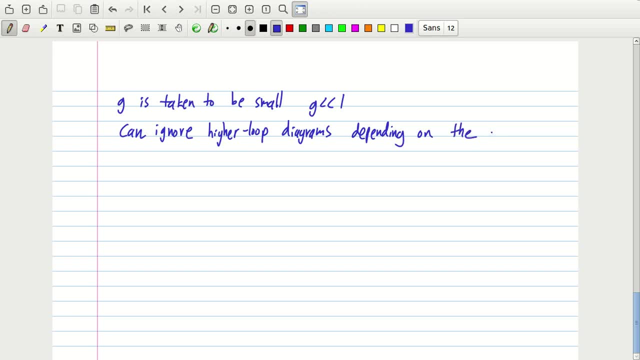 on the, let's say, resolution we are aiming for. Okay, so basically, how accurate do you want our answer to be? Of course, the more diagrams you include, the more you get closer to the correct answer, which is the blob. 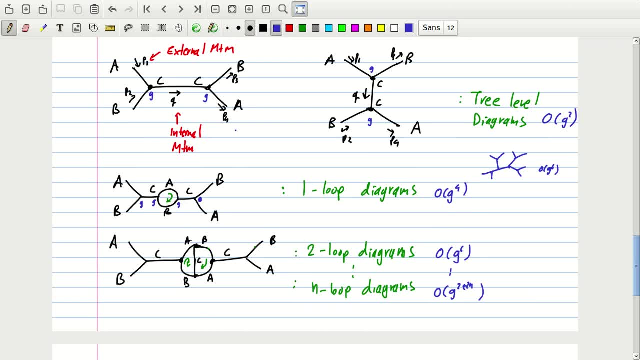 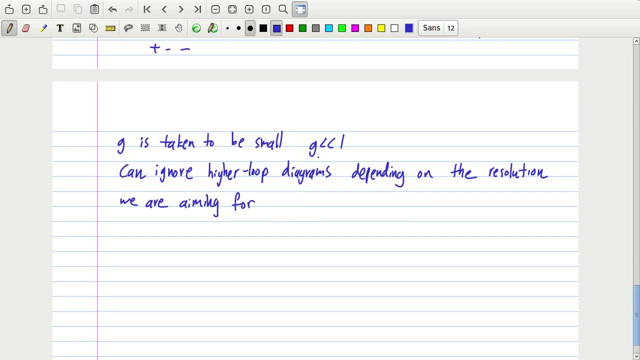 This is the full answer. So these are all approximations to the blob. because you're just, you need to add all of them to get the blob. But if g is very small, you can get away with ignoring it because eventually, 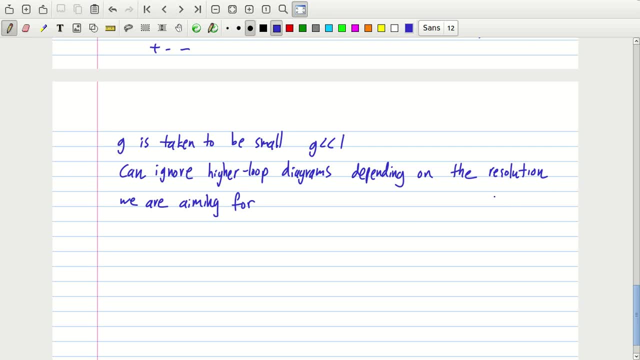 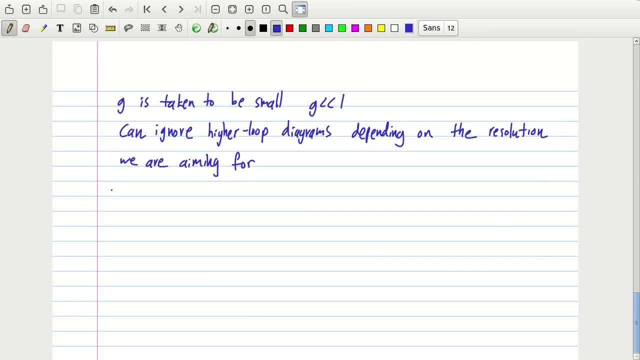 you're going to end up adding all of these extra diagrams, It's going to give you some correction to some decimal digits, because g is very small. So that is the essence of what is known as Feynman perturbation theory. 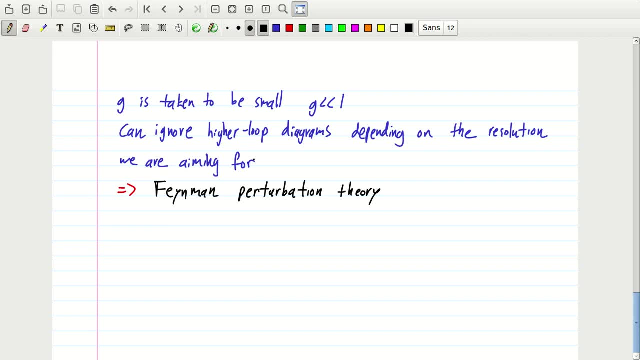 Okay, so basically, you don't need to add everything You ignore. you work with specific at the specific loop order, So work up to a specific loop order. Okay, so we're not going to go into all the details, but you can definitely check. 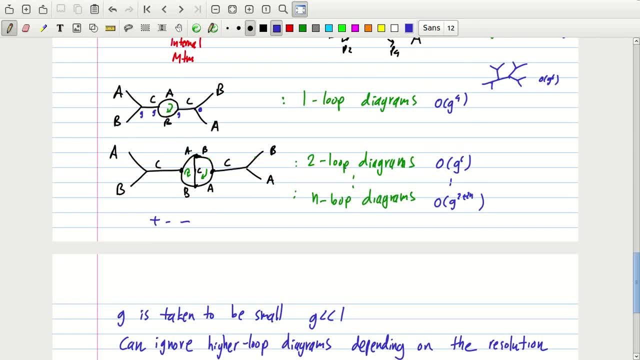 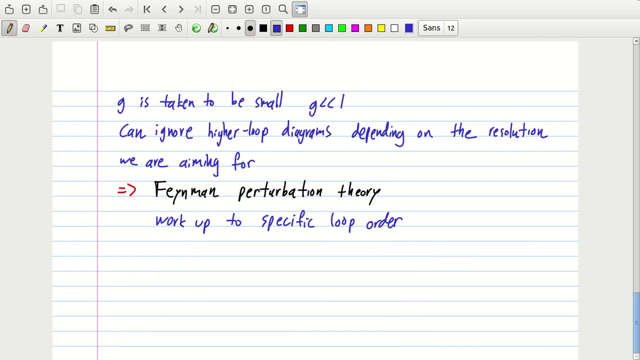 I already did this for zero, one and two loops. You can verify this formula that I wrote by drawing some you know six-loop diagram. seeing does the formula still work for g? And we're basically done, because this is all. 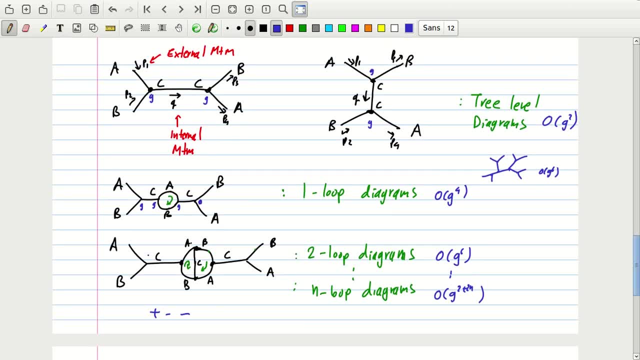 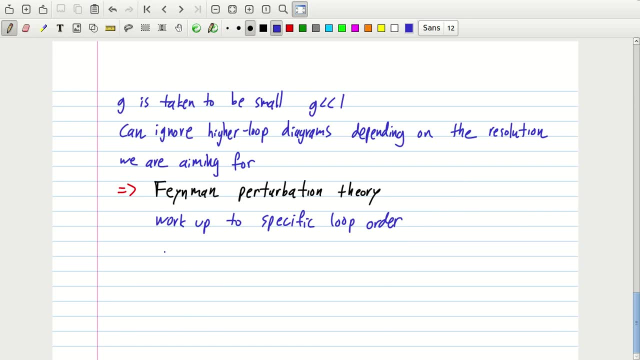 that Feynman rules, or this is actually the main step of the Feynman rules, which is to write down the diagrams corresponding to a given process, But now, of course, okay, there's a bit more to it that we need to. 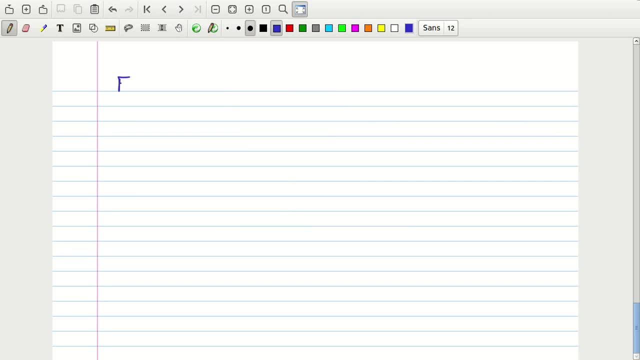 just quickly go through. So the Feynman rules tell you more specifically how to draw these diagrams. Now, once you've done this, basically add these and draw these diagrams. what do you do with them? So we need to first associate. 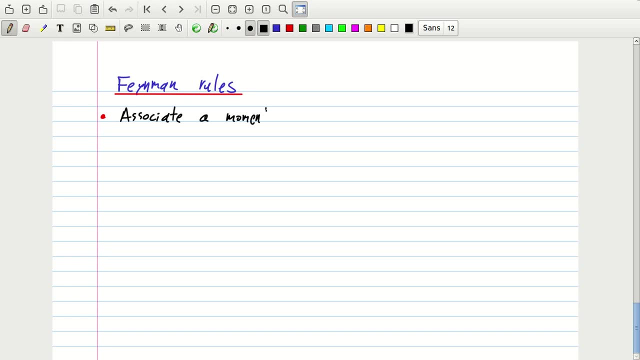 a momentum to each line in the diagram. Now I'll show you how to do this. You can see that you can actually use this with an arrow. Okay, so it's. so. of course, it'll need to have a particular arrow. 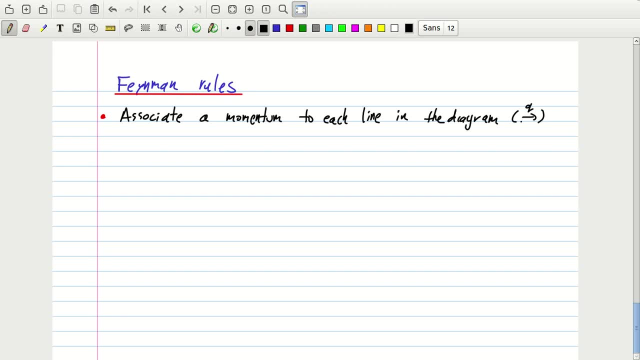 depending on- Now it's kind of arbitrary- which way the momentum is pointing. The rules actually take care of the direction, but you need to choose an arrow for each momentum, Okay, so if you have your, say, your one-loop diagram. 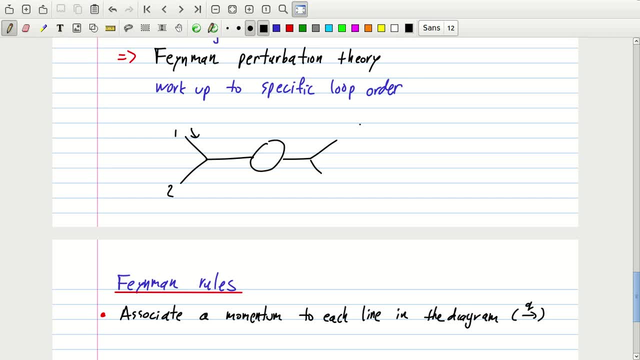 now you need to choose. Now you need to start putting momenta P1, P2, now we can call this maybe Q, Q1, Q2, Q3, Q4, and then the external momenta, again P3, P4.. 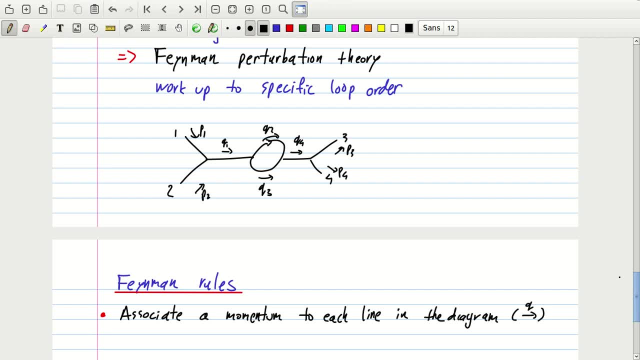 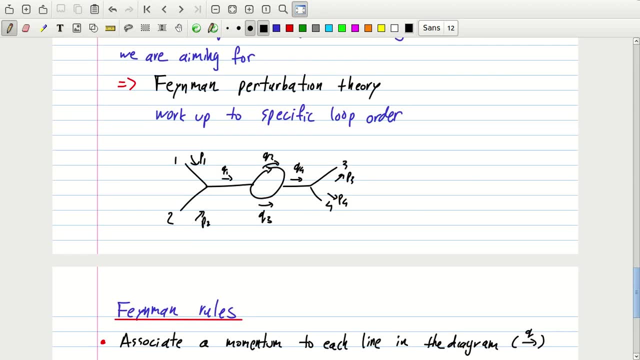 Okay, so we need to put all of these momenta for each line in the diagram And I will be using Q for the internal momenta. There are different sometimes. they are often called K as well instead of Q. I think maybe in my notes actually I'm calling them K. 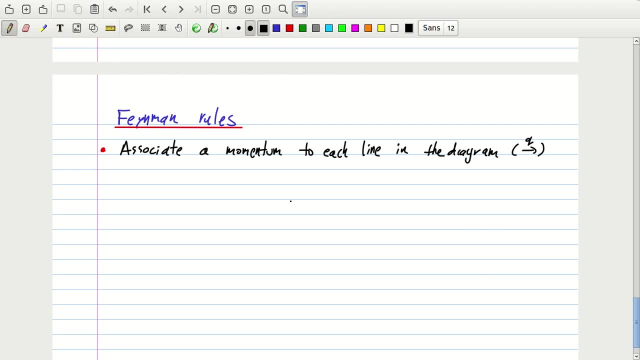 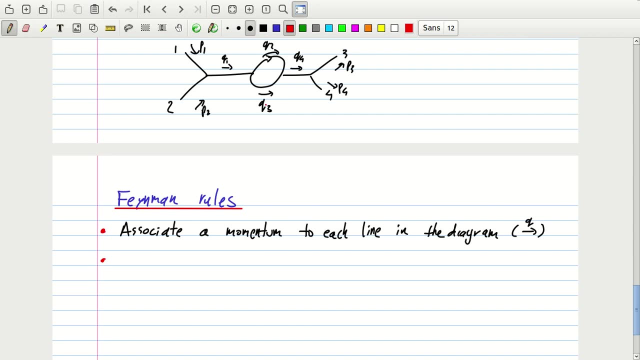 But okay, so that was easy. You just write down a momenta in any direction you like. Now, as I emphasized, I could have written this Q3,, for instance, pointing in the other direction. It does not matter in the end in the rules, 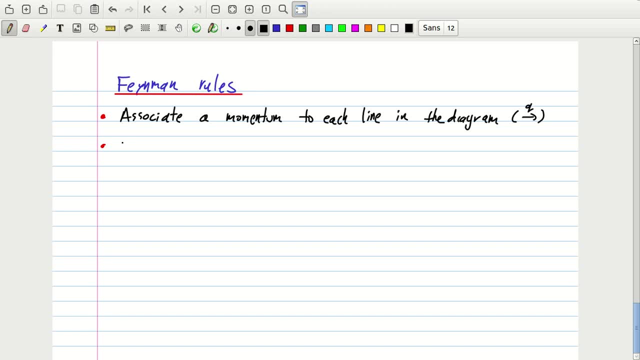 For each vertex we need to include a factor of minus i, g, 2, pi to the 4th, And a delta function. so a four-dimensional delta function which is the sum of K, which are the momenta that are entering the vertex or leaving the vertex. 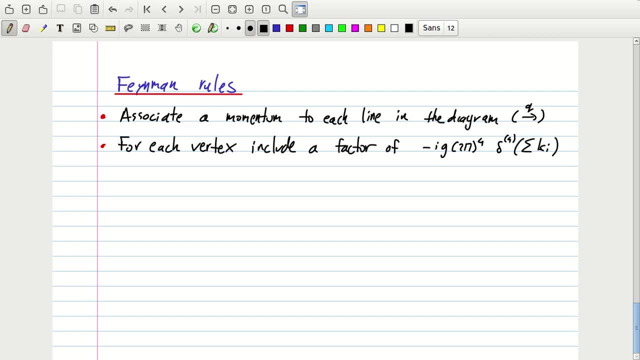 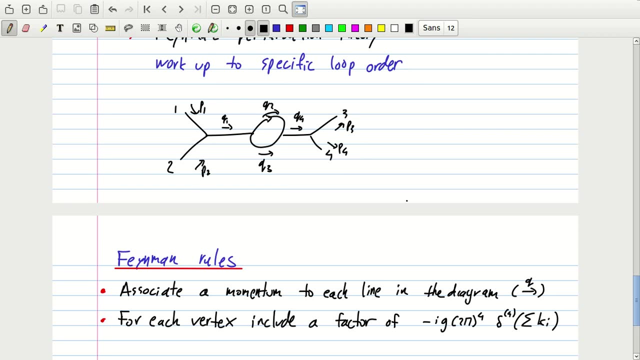 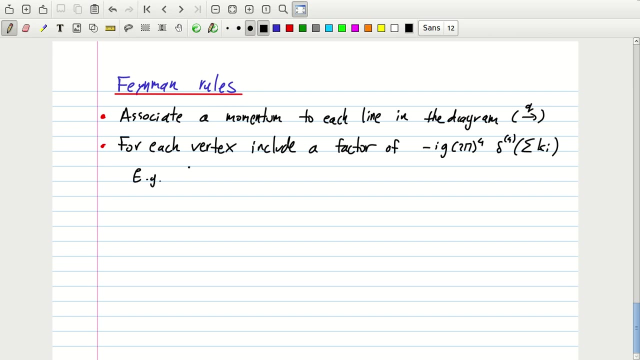 So if you look at, if you look here, there are two momenta- P1 and P2- entering and one momentum leaving. So you would write Eg, we would write a delta of P1 plus P2 minus Q1 at this vertex. 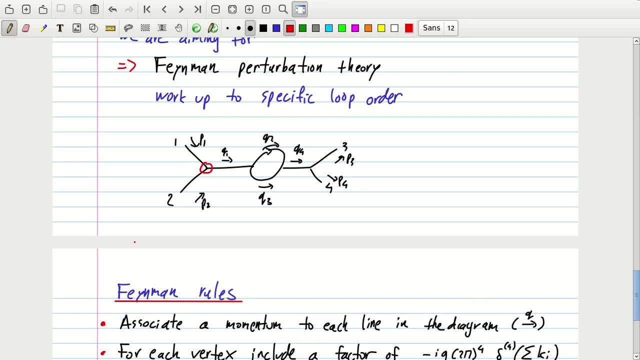 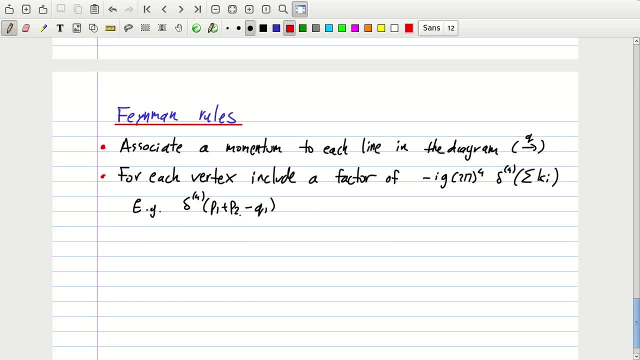 So at this specific vertex I'm looking for, you see that there are two momenta- incoming and one outgoing, And if it's outgoing you put a different sign. So you would write something like this, Or you would write: if you look at this: 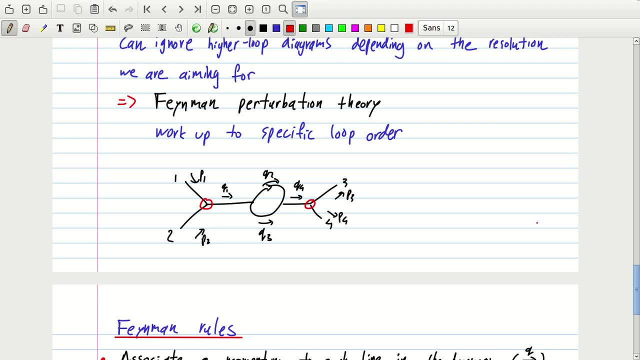 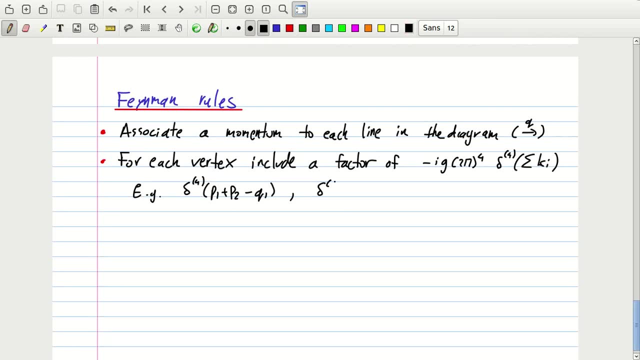 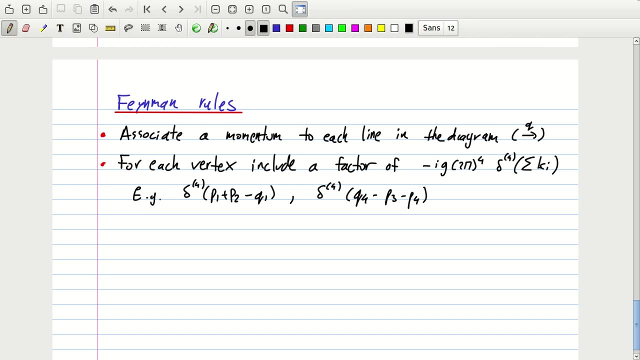 At this vertex there's one incoming momentum, which is Q4, and two outgoing, which are Q3 and P4. So you would write delta to the 4, Q4 minus P3, minus P4. And so on. Okay, so you can do the same for all of these diagrams that we had earlier. 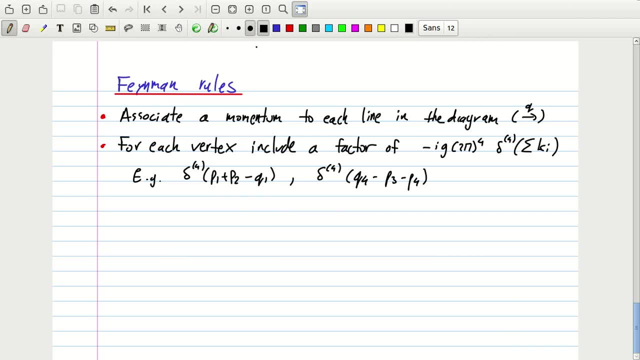 So that's the next rule, Now for each line. By the way, I'm not Going to really ask you to memorize all the rules. This is just to try to understand somehow a bit that there's something behind all these diagrams. 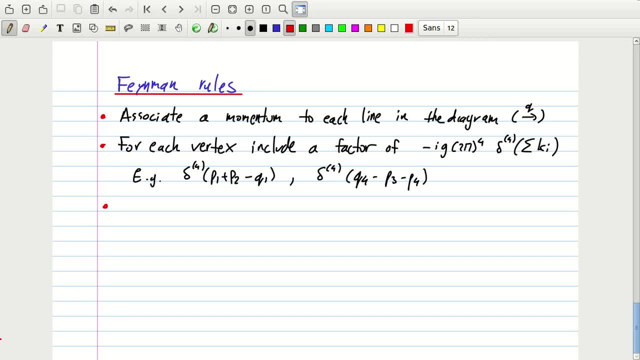 that they're actually corresponding to specific. I mean, there are prescriptions for calculating an amplitude, So I'm just giving you the prescription. But what I'll mostly be asking you is to be able to draw the diagrams, To understand how you get all the different diagrams, and not so much applying the rules and getting the final. 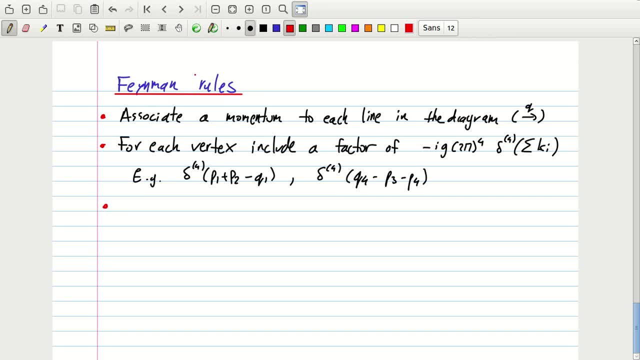 So for each line in the diagram contributes, Contributes, a factor of I over the Q which corresponds to this line. This is the internal line. Sorry, maybe The internal contributes a factor like this: M is the mass of the particle of which corresponds to that line times a differential. 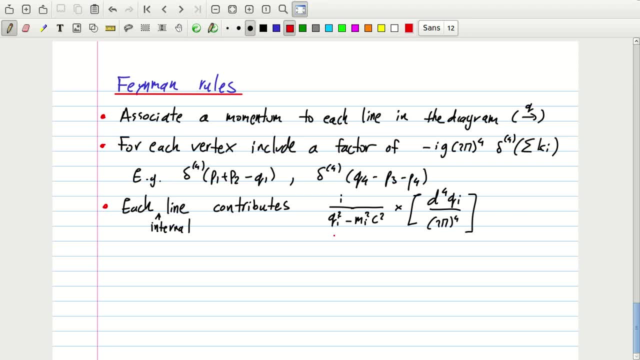 Like this. This part, just for notation, is called the propagator And a large part of the say the QFT course. Well, there's a significant part of the QFT course which deals with how to calculate this propagator. 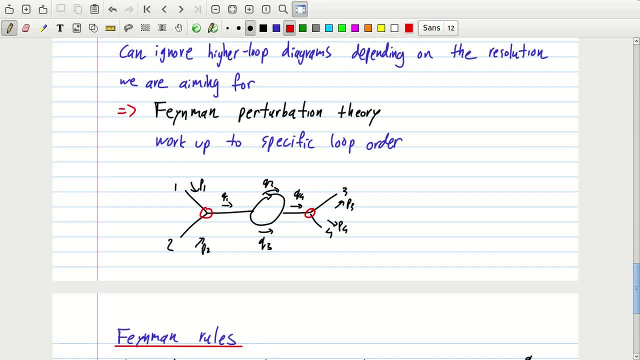 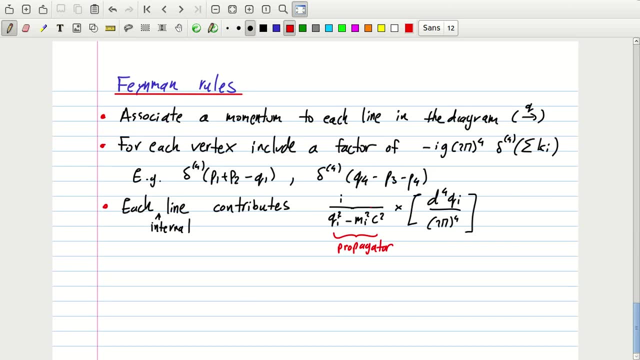 Like: how wide is a propagator? What? Why does a line get associated? So this is this line that I drew here. You need to associate each of these lines with this kind of factor. Okay, so to understand this, you need some work that needs to be done, which, of course, we're not going to do. 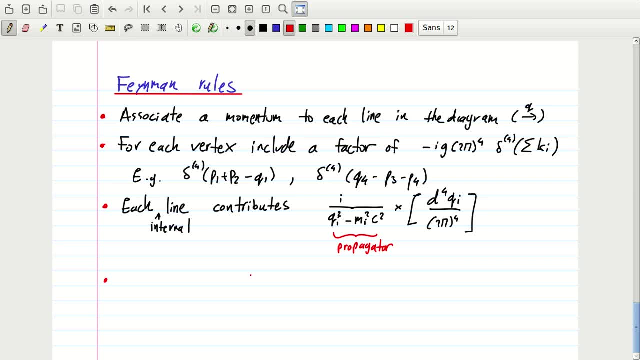 So we're not going to do that, We're not really doing it at the moment. Okay, so there's just a statement that you need to add this, And it tells you basically how the particle travels between when it's created and when it decays. 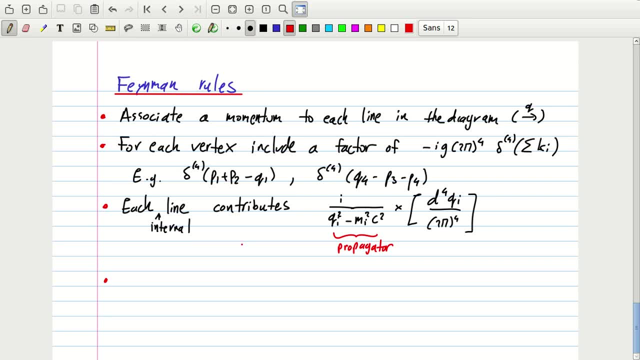 Because an internal line is always created somewhere and it decays somewhere else. It's destroyed somewhere else. So the propagator tells you how it travels between these two points. Now comes the crucial part. We need to integrate over all internal momenta: QI. 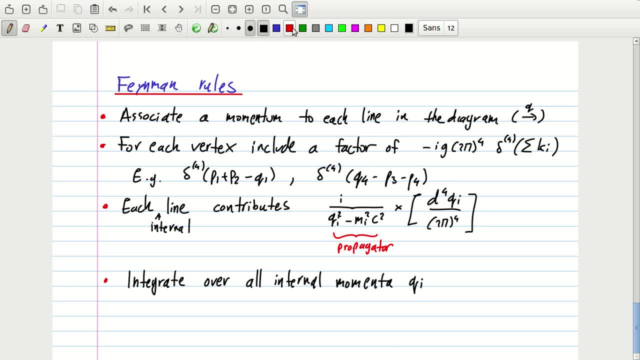 Okay, so you have these factors of d for QI. So all this rule says is: well, add the integral sign. Okay, so now actually integrate over all of these. Okay, Okay, Okay, Okay, Okay, Okay, Okay. 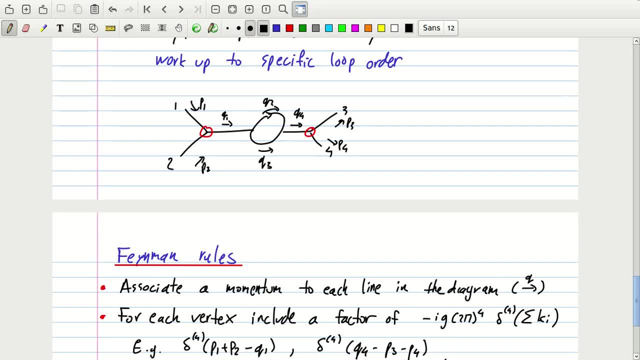 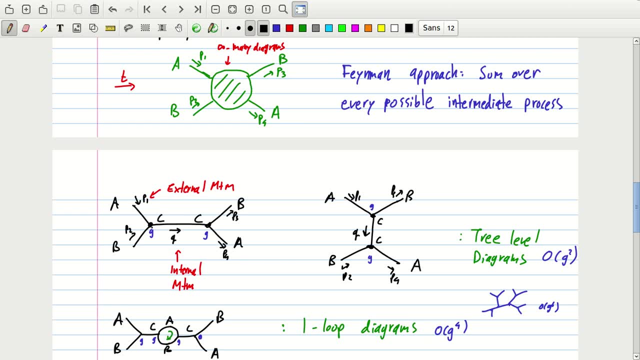 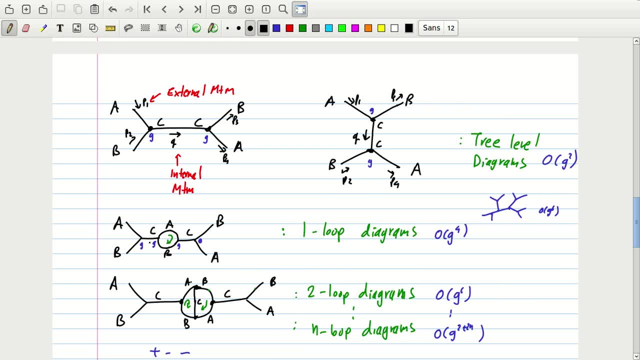 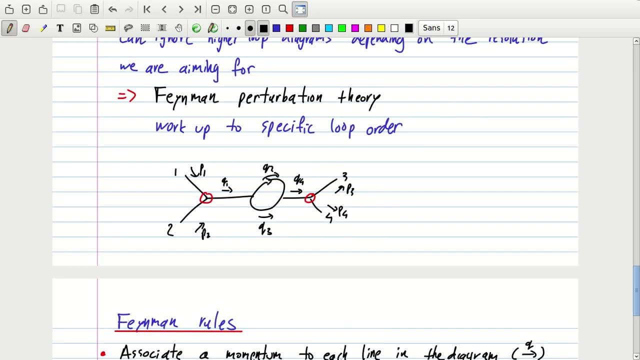 If you have a one-loop diagram, you have one, two, three, four Qs. Actually I wrote them here: One, two, three, four Qs, So you have four integrals. Okay. so the number of integrals goes up very quickly with. 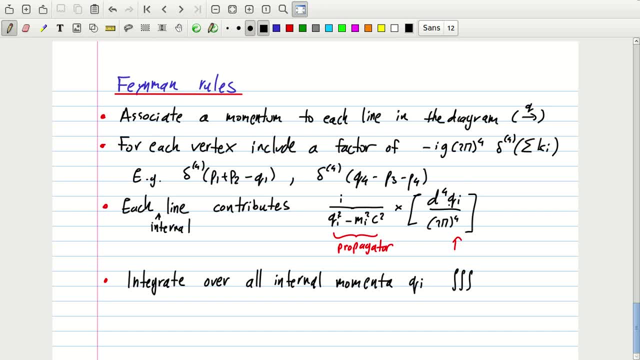 the level of the diagram, And these, of course, are four-dimensional integrals. Now this should- and we'll see an example now- that should give an overall. I mean, apart from many other things, it should give an overall factor: delta 4. 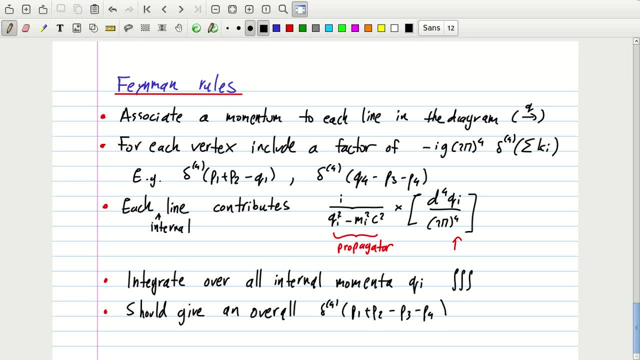 p1 plus p2 minus p3 minus p4 for the four-dimensional, for the four particle scattering we were looking at, If you had more particles you would get the correct delta function, energy-momentum conserving delta function for those numbers of particles. Now this: 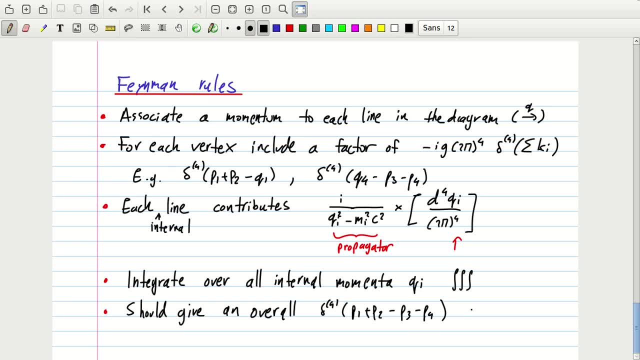 already. there is already there in the Fermi golden rule, so we remove this Remove because it's already present in the Fermi Okay. so this is a bit of an embarrassment. one could say that, okay, you get the same delta function in two parts once you get it by the Feynman rules. 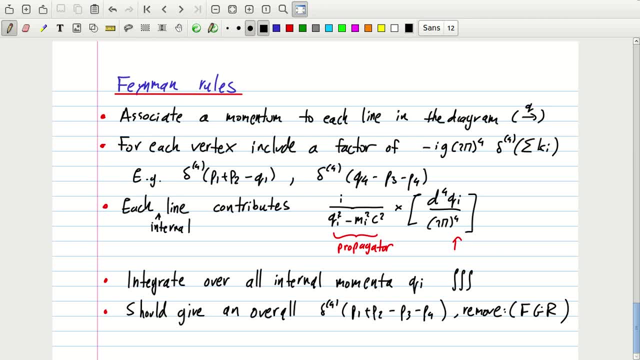 and once you get it from the Fermi golden rule. But remember, these are formulas that are meant to be practical and to work and they definitely work. So you admit a little bit of redundancy in the formula. let's say, getting the same delta function twice. 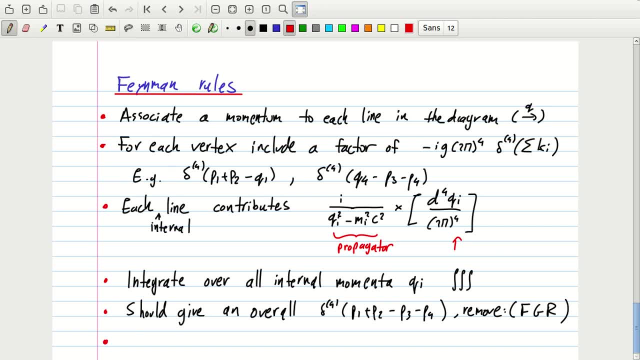 And what you get after you do. all these integrals should actually be minus i m, the amplitude, and if you square, you get the m squared which enters the computation of the cross-section, And that's it. these are the Fermi rules, at least for this theory. 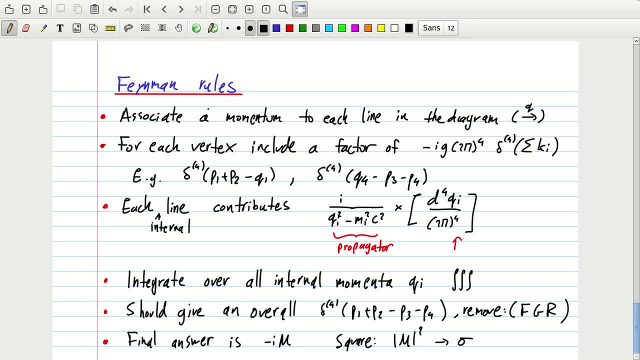 Now, if you were to go to a more complicated theory, which was not just abc, but more complicated things like photons and electrons, then some of these steps would not change at all. So step one and two will be exactly the same, because they still carry momentum. 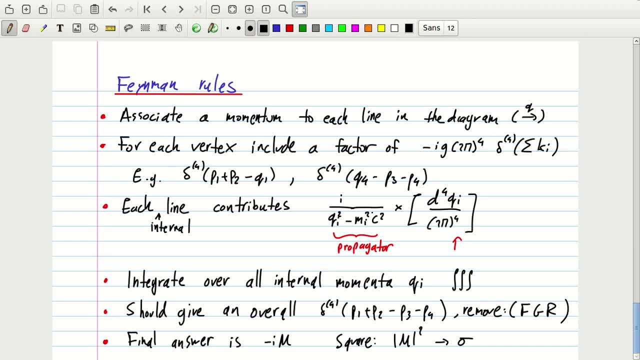 but the propagators will be different And actually the vertices will be different, So that the sum of momentum is going to be fine, but the actual vertex will be different for different particles And the vertex might actually- and that's a major complication- 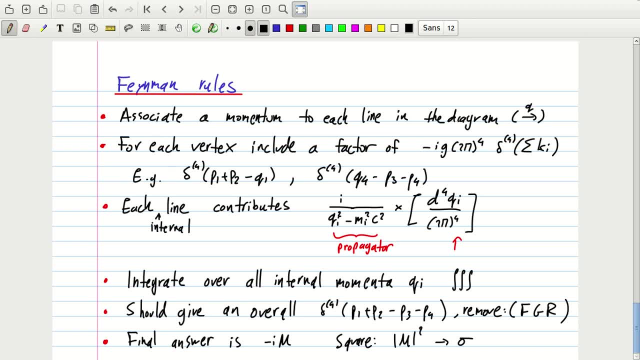 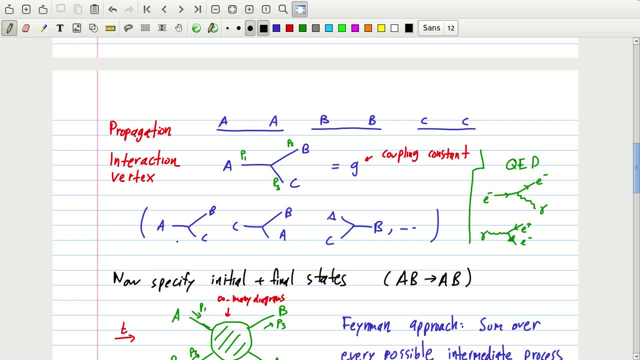 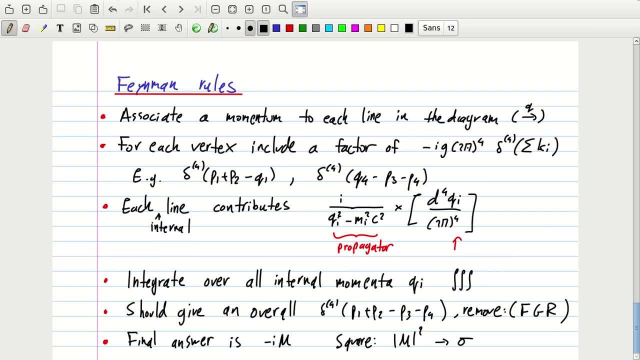 might depend on the momentum of the particle, And you might also have vertices which are not just simple vertices like these. you might have more complicated vertices which, for instance, include four particles. So things, of course, are going to get more complicated both with the vertices, not the momentum. 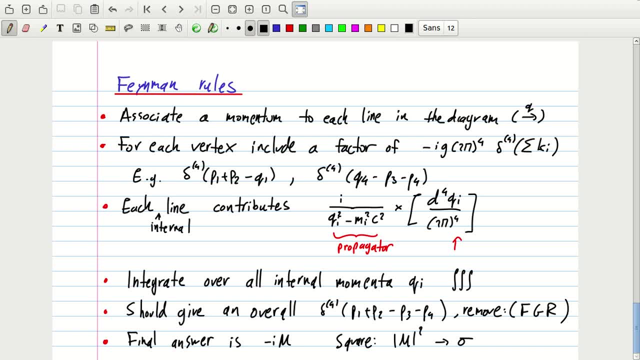 the momentum is always kind of very similar, the way you deal with them, but the actual what you put as a vertex might be different. which vertices you are allowed, so what graphs you can draw, are also different, And the propagators are different. 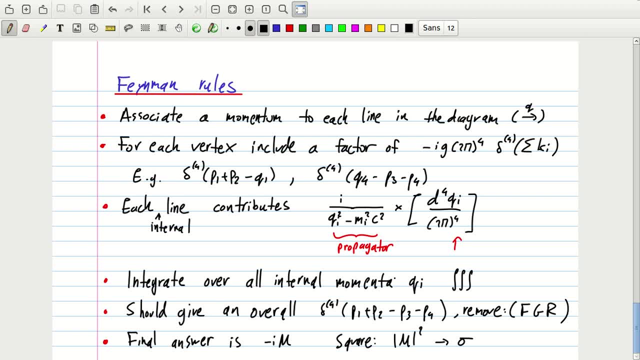 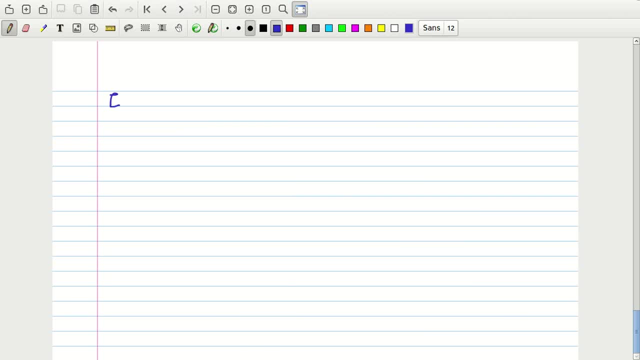 And to account for things like spin and so on, But these are the essential rules. So let me end with a little simple example of how you apply these rules. For instance, let's do the simplest possible thing you can think of, which is that you have an, A particle. 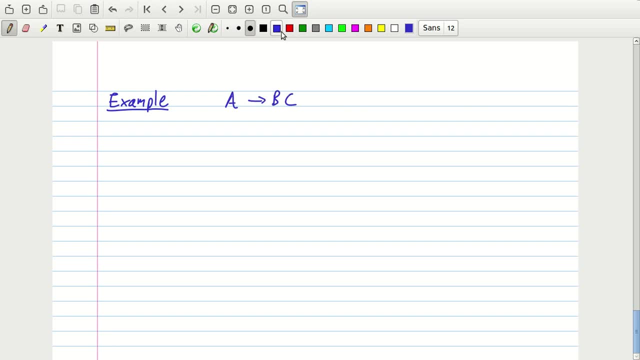 which splits into a B and a C particle. That's an allowed process. So the diagram would look like this And we'll put the G here. So how do you apply the Feynman rules here? In this case? there is actually no internal line. 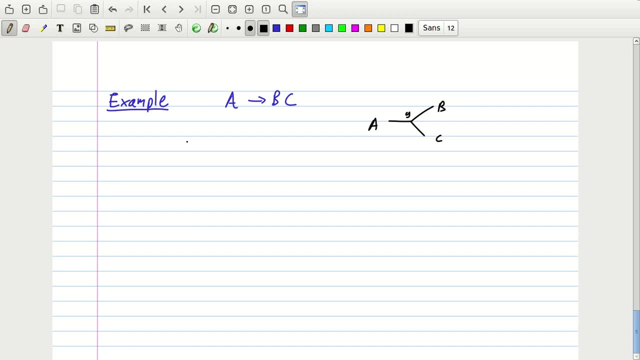 So for this vertex you would need to put a delta function of delta 4 of P1, P2, P3. So you would write P1 minus P2 minus P3. But this is something that we need to remove, because this is exactly what is there in Fermi's golden rule. 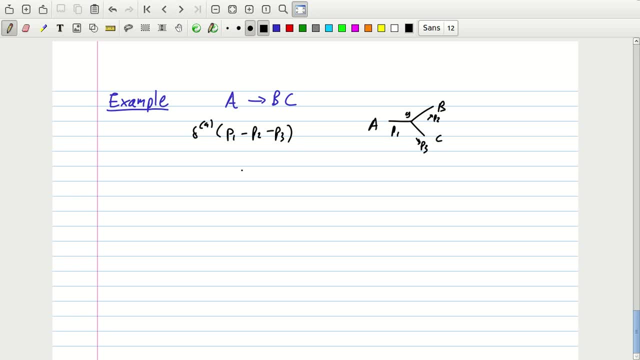 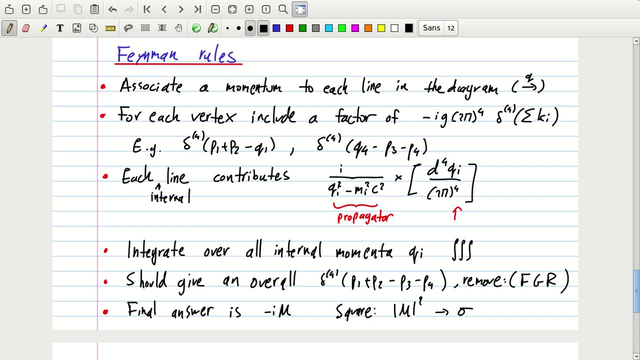 And now, if you go back to the previous lecture, well, basically the amplitude. sorry, let me write it like this: The amplitude. if you write it carefully, if you look at all these processes, there are no propagators, There's only this. 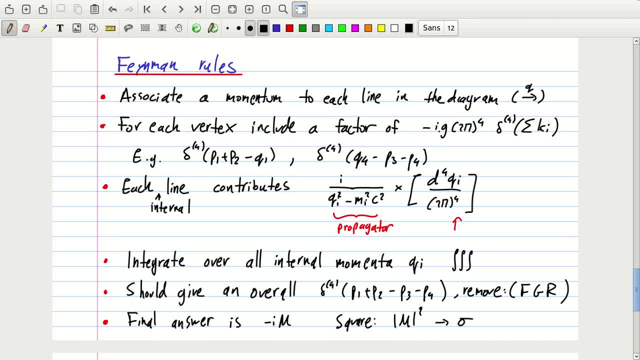 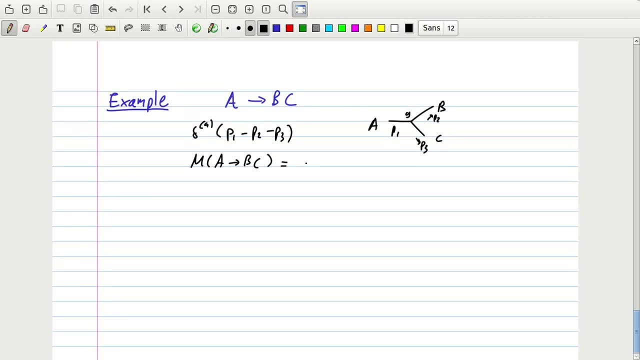 So you would get something. you'd basically just get this minus Ig 2, pi to the 4.. But roughly what you get is G up to maybe some factors of i that are not important because we're going to square it, So squaring this. 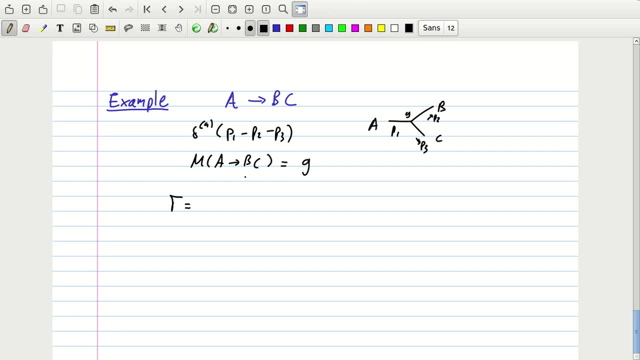 we can get the cross-section, because now you need to add all these other factors from the 1,, 2, 3 decays, for which you need to look at the previous lecture. But you square this and you get that the amplitude is proportional. 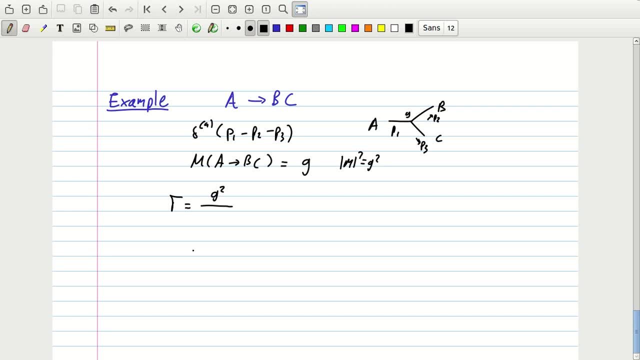 sorry. the decay rate is proportional to G squared And if you put the correct factors you get something like 16 pi H bar times the mass of the A particle And we. this assumes some things like B and C being massless. 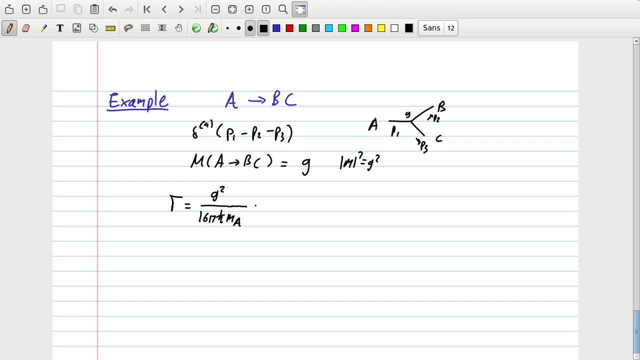 So there's the momenta. there are no momenta there and all that But this. so there's no masses of the B and the C, But that's roughly how you'd get it. So this is a very simple case where you apply the Feynman rules. 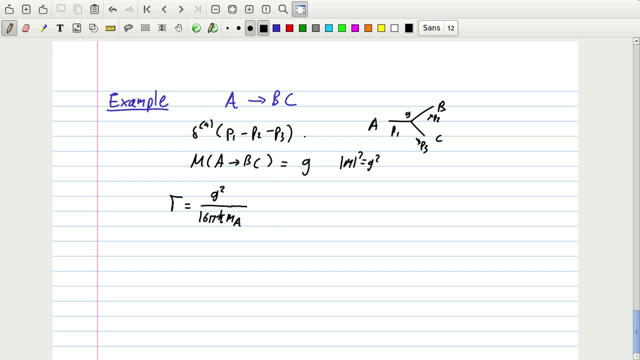 and you don't get anything special happening. But suppose we go to the next, more complicated example, which is say A, B, giving you A B as we had before. So we draw. I'll just emphasize one thing: I want to do the full computation. 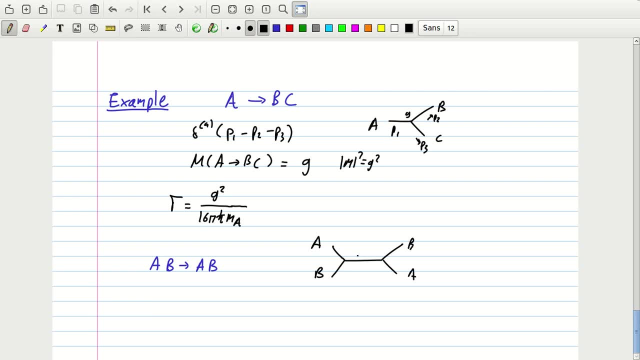 A, B, B, A. remember here there was a C which carried momentum Q. So now we need to do roughly without really doing all the, without keeping all the factors you need to integrate over Q. There is no QI, just one Q. 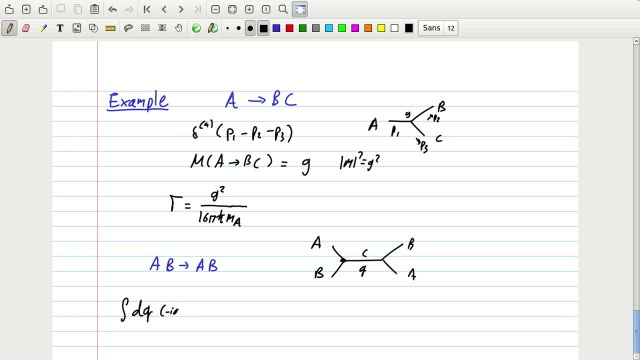 This vertex is going to give you a factor of minus IG delta for P1 plus P2, minus Q, So again 1, 2, 3, 4.. So that's called P1, P2, P3, P4. 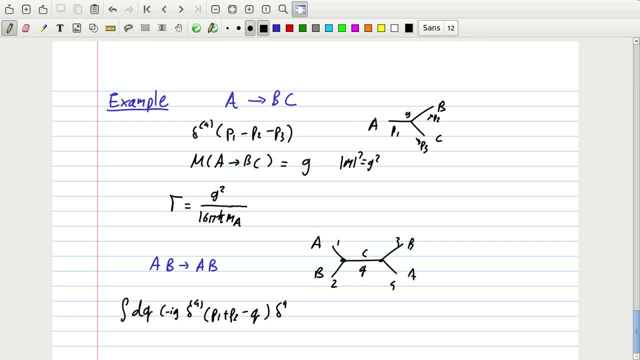 This vertex is going to give you a delta for, as we saw before, Q minus P3, minus P4. But now you're instructed to integrate And there's one integral you need to do over Q. Again, I'm skipping all the factors. 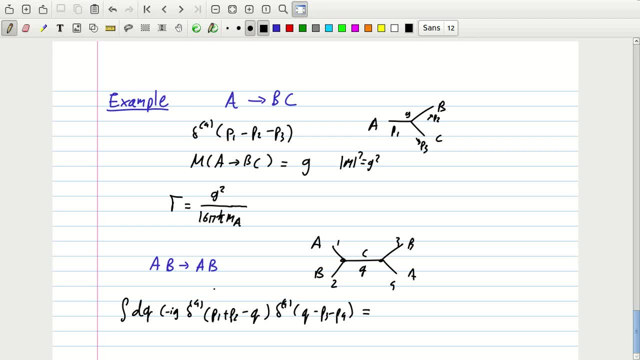 But what does this tell you? In integrating, you can use one of these delta functions, For instance, you can use this one to do the integral, And you what you get is that this forces Q to be equal to P3 and P4.. 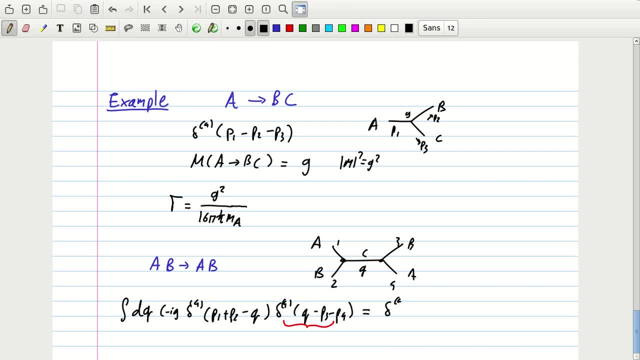 So, after doing the integral, you end up with a delta function which is P1 plus P2, minus P3, minus P4.. And that is exactly the overall delta function that we said you should get from here. So again, in this case, 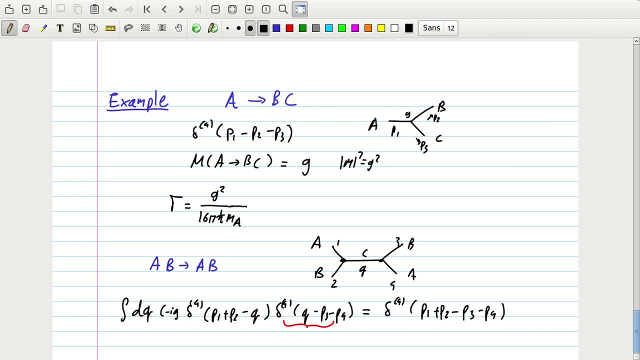 there is no real integral to do, because you only have one integral and you can always do one integral because of your delta functions. Now, in practice, what will happen is, if you go to loop diagrams and you try to do these integrals, you will have more vertices. 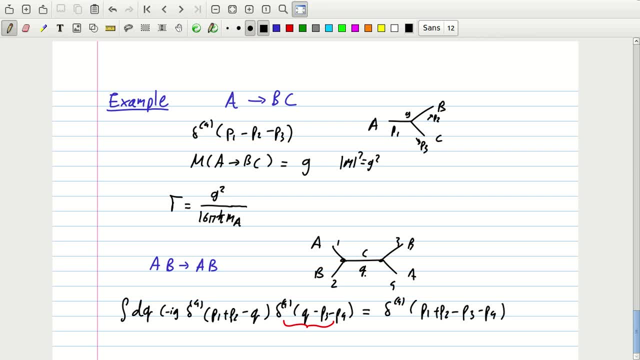 than your corresponding momentum. So you're not going to be able to integrate all of them using delta functions. There's going to be some integrations left over for you to do, which, as I mentioned last time, is where the complications really are. 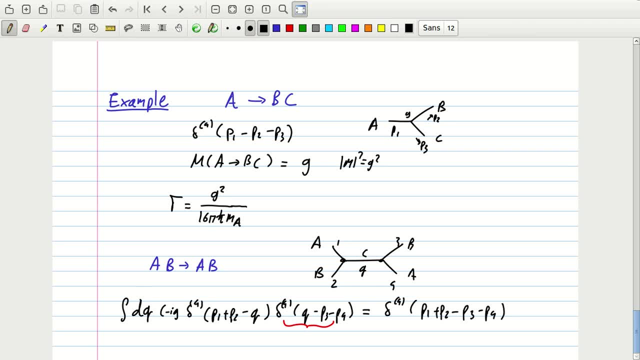 technically, These are complicated integrals that you're going to need to do. I'm not going to ask you, of course, to do these integrals at this stage, because I'm not really developing the theory fully, but I think it was important. 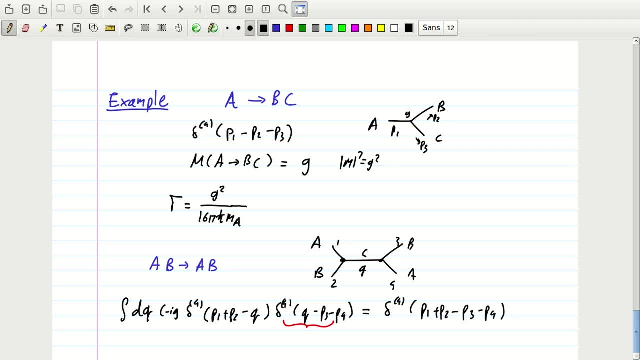 to just give you this overview. So we're going to do maybe a couple more examples of how to find the graphs, the Feynman diagrams at higher loops, just to make sure that we're not missing any diagrams, and maybe I'll clarify some more things. 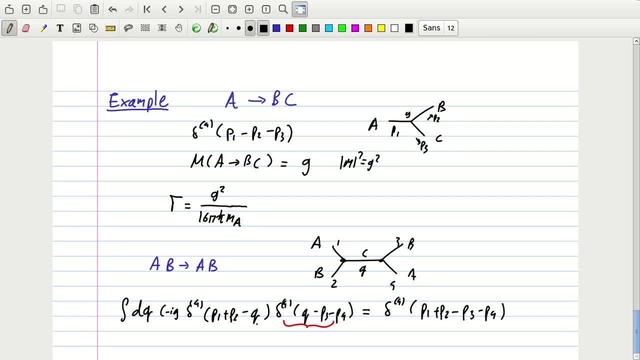 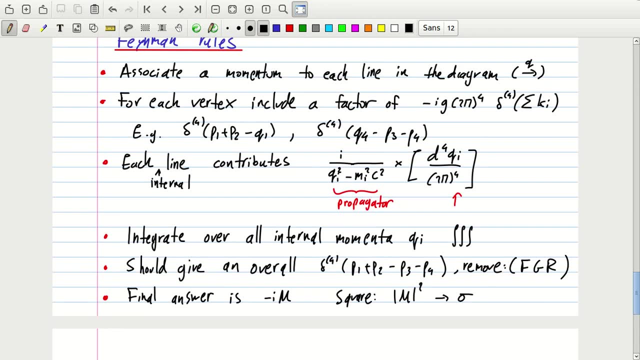 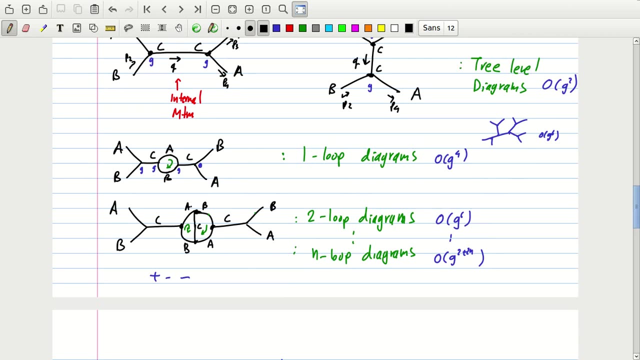 about how the integrals work for the loop diagrams, perhaps in the next tutorial. But what you need to know is basically just have an overview of these rules and basically get some practice with constructing one loop and two loop and so on diagrams, depending on the process. I ask you. 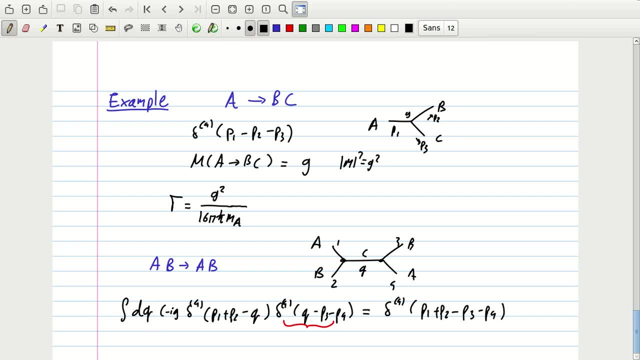 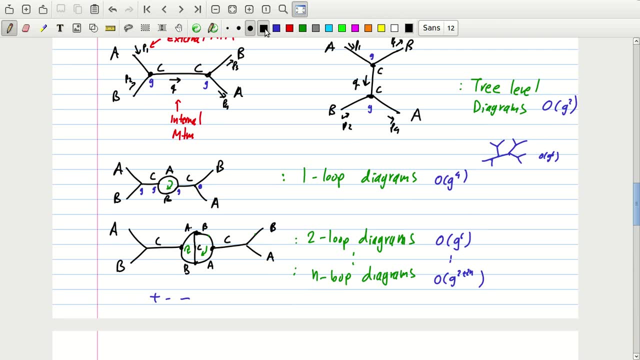 Okay, So you have to remember that different processes can lead to very different diagrams, For instance, what I was trying to do here. you could write a box diagram like this, but only if these are all Cs, for instance, So then you could write A, B, A, B. 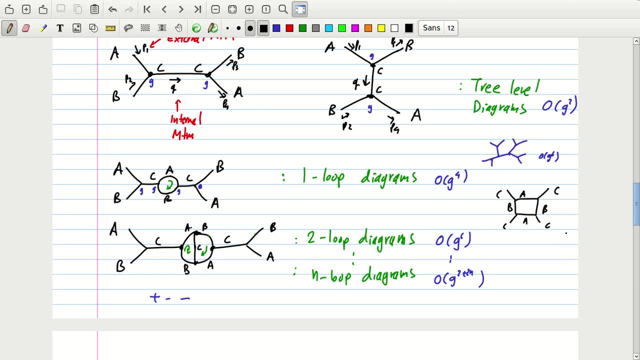 So in that case you could definitely write such a diagram, and that will be different from Then. you would not be able to write diagrams like these, because a C and a C cannot be next to each other. but here they're not.